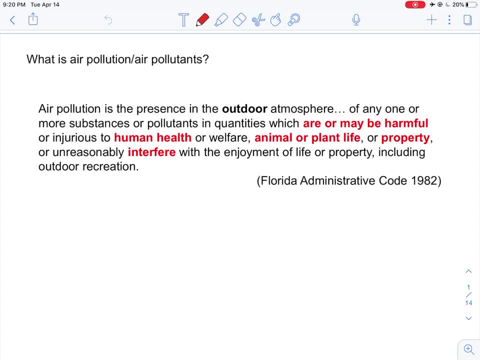 Sometimes you can smell some really strong acid smell. Those might be sulfur dioxide or nitrogen oxides. So you can see that these things are different And typically you have a feeling that there are kinds of hazardous in the environment, right? So according to a more complete definition of the air pollutants- and actually I pasted this sentence here- 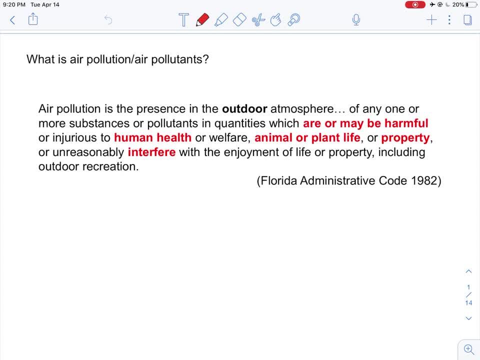 This is coming from the Florida Administrative Code in 1982.. So the air pollution, according to their definition, is the presence in the outdoor environment. So please notice that right now we're just mentioning or we're talking about air pollution. We're just talking about the outdoor environment. 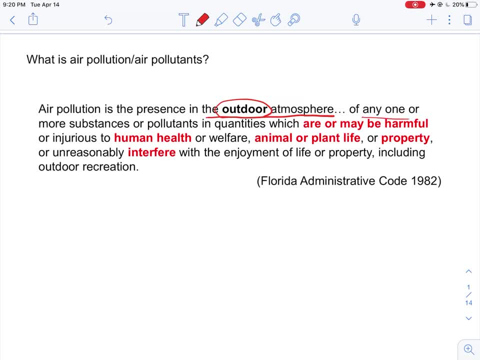 So it's the presence of any one or more substances, So it's not limited to one type of the chemicals or pollutants in the quantity which they are or may be harmful. OK, so you can see that they can be harmful, or even if we think that they may be harmful, we'll still categorize them as the air pollutant. 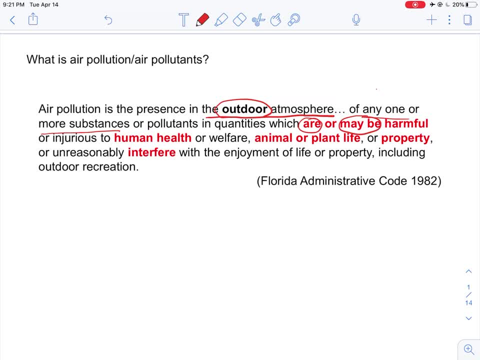 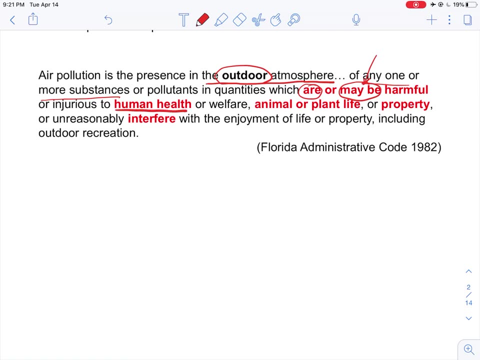 So I'll introduce more background on why sometimes we can put some doubts or put some discussions on the air pollutants that are maybe harmful. OK, so they can be harmful or injurious to human health, right? Because when we see dust, when we inhale them, they are going to be harmful to our respiratory system. 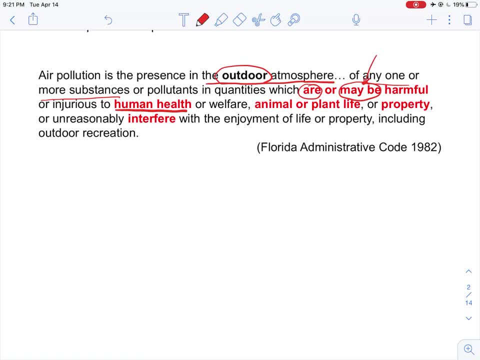 And for those gas species that have odors, they're also harmful to our respiratory system. right, It's going to harm our human health, So they can be also harmful to the welfare or animal or plant life or properties. OK, so you can see that when we categorize something as the air pollutant, it's not only affecting our human health. 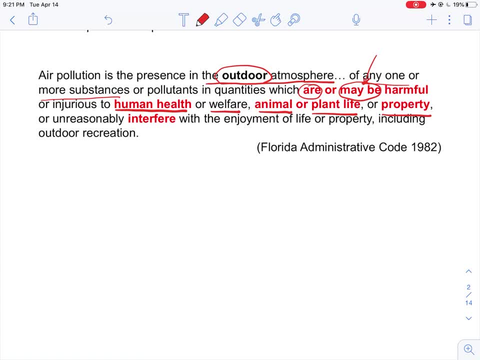 So if they are affecting any one of these, we can categorize them as air pollutants, right? So not only these, they also include something that's unreasonably interfere with enjoyment of life or property. So we're talking about air pollutants. 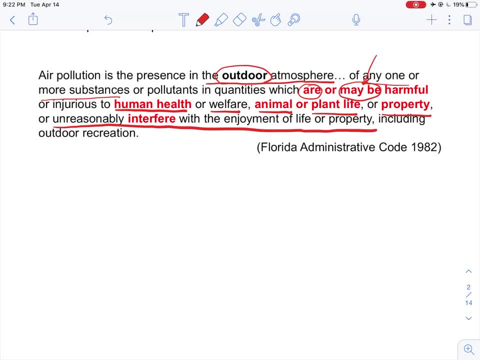 We're talking about a broader feeling or broader definition of the air pollutants, right, Including the outdoor recreation. So even if they're not harming our health, not harming the welfare, not harming the animal or plant life or property, as long as they unreasonably interfere with our outdoor activities or enjoyment of life, we can say that that is an air pollutant. 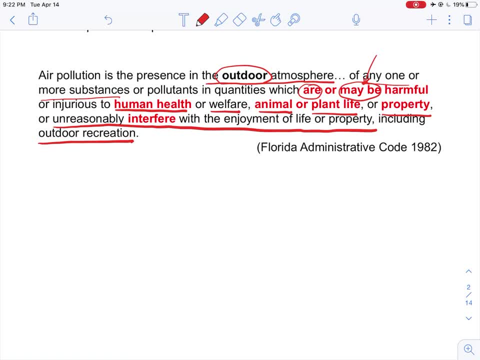 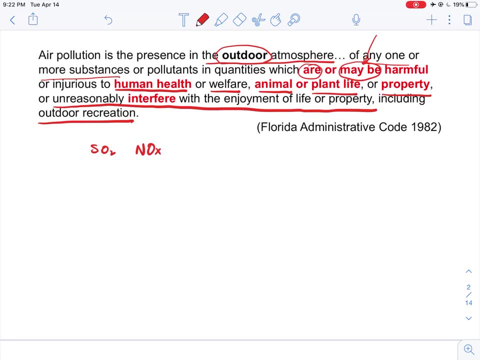 So by seeing this definition, what I mean is that, for example, if we're talking about the sulfur dioxide or nitrogen oxides, OK, so typically we'll use NOx. So maybe mainly because NOx includes nitrogen monoxide and nitrogen dioxides. 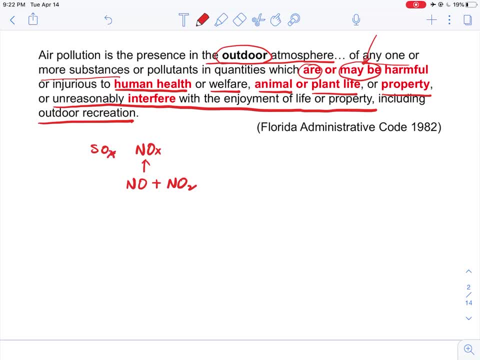 OK, so because of that, we can also show the sulfur oxides as SOx, because the SOx includes sulfur dioxide or sulfur trioxide, So they can co-exist in the atmosphere. OK, so let's say that the SOx or NOx, they can be emitted in really far away distances. 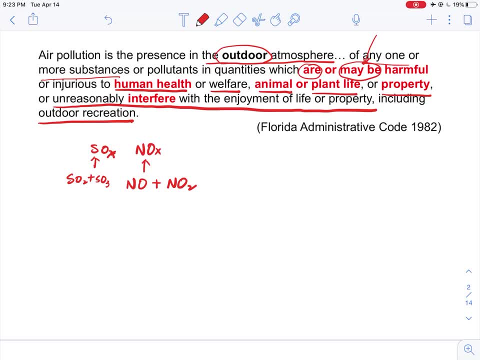 Let's say they're emitted in a location that there's no human being living nearby or no animals living nearby for around it for 10 kilometers, right? So even under that situation, we can still categorize them as air pollutant, mainly because once they're emitted into the atmosphere, 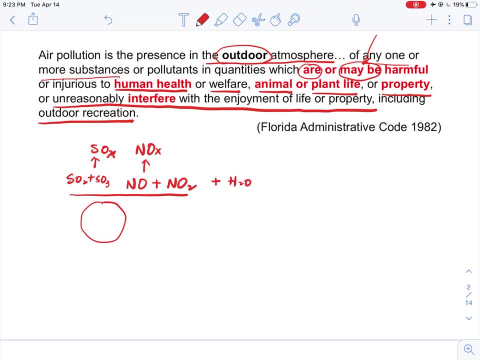 they have the ability to form acid rain right. What that means is they can basically combine with the cloud droplets that's suspended in the air. So, for example, this is the ground right, And then this is a plant that we're talking about emitting the sulfur oxides, or nitrogen oxides. 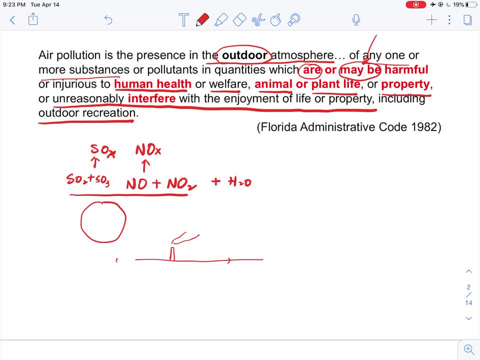 So even there is no human living nearby. So once they're emitted into the atmosphere, we sometimes a lot of time we can see clouds there. So these models, they're very similar. So these molecules can combine with the cloud droplets that are in the clouds. 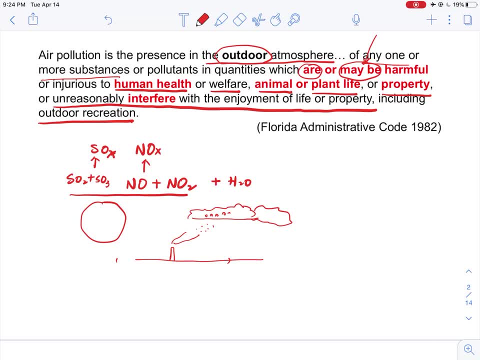 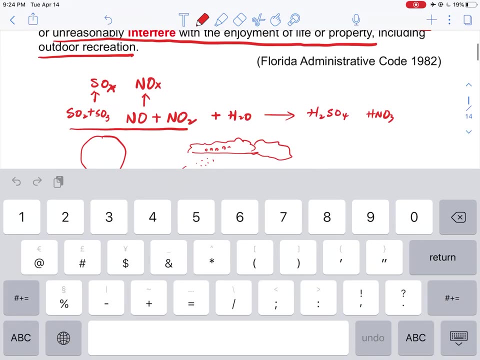 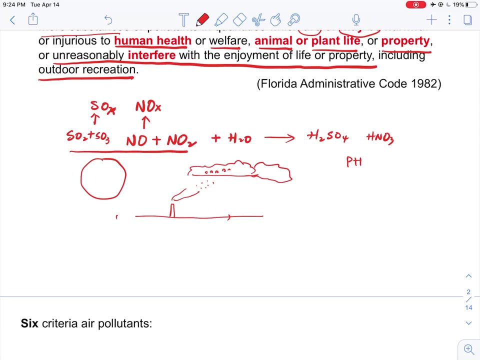 And we know that cloud droplets is mainly composed of water, right? So once they react, they can form sulfur or sulfuric acid or nitric acid. right, We know that these acids have a very low pH, right So once they have a low pH, which means that they have a high concentration of the protons, 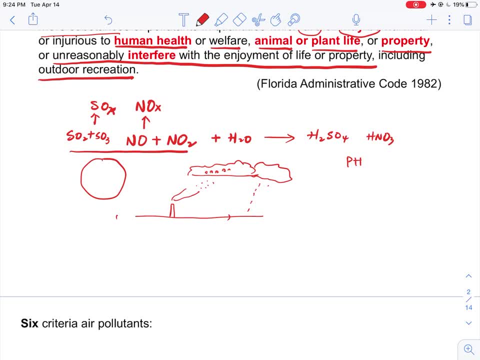 So once they form rain, they don't necessarily have to form rain nearby the plant here So the rain can be formed, let's say, hundreds of kilometers downwind of this plant here, So that's going to harm the life or the human health or animal or plant life, so on and so forth. 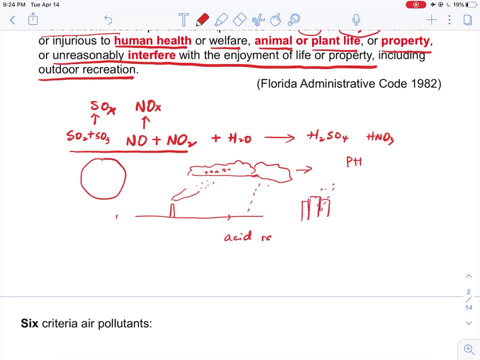 So we don't like the acid rain, mainly because, for human, we can just hold an umbrella to stop the rain from falling onto our body right. But for a lot of the constructions or sculptures, we know that there are a lot of famous sculptures that are designed by human right. 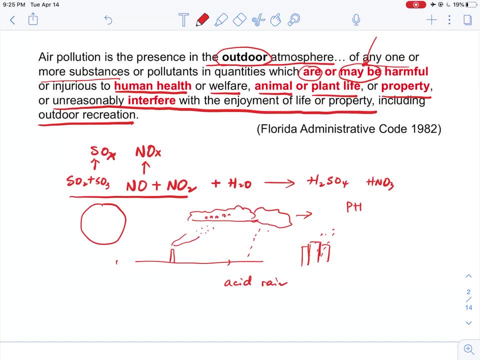 A lot of them exist in Europe and other parts of the country, other parts of the world. So once this acid rain drops onto these constructions or sculptures, we know that their composition is mainly metal or calcium carbonate right, And we know that the calcium carbonate can be reacted by these acids. 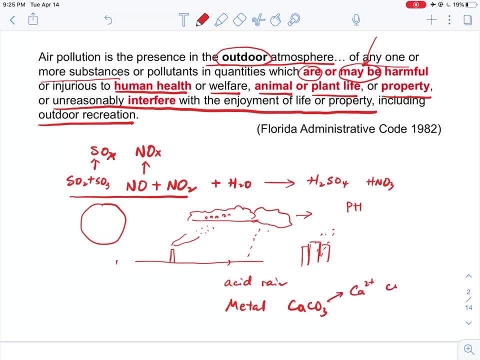 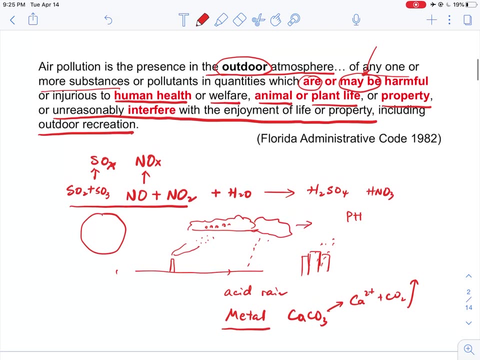 basically form calcium ions and carbon dioxide, right? So that's going to corrode all of these constructions or sculptures. So the same will happen for the metal, because metal are much more easier to react under this condition. okay, So this is a more complete definition of the air pollutant. 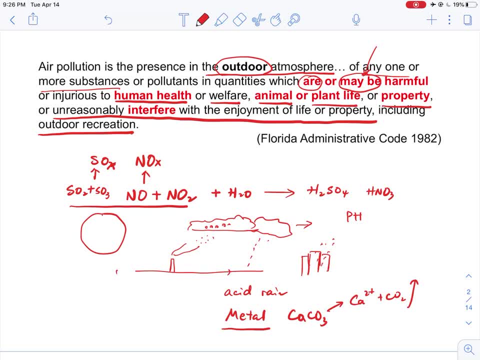 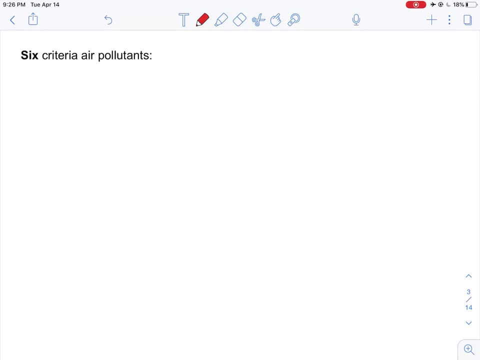 So you can see that there can be a lot of different types of air pollutants, right, Because we're giving you a very broad definition of these air pollutants, right? So, in terms of the air quality control or the air pollution control, we're mainly interested in six criteria: air pollutants: 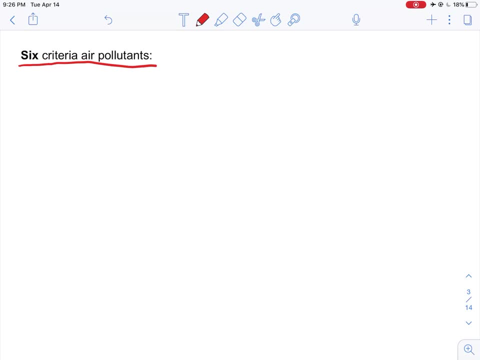 So what that means is that we're interested in six most important air pollutants. So they're important not only because of their toxicity. right, We have to say that these air pollutants have to be toxic, Otherwise, if it's beneficial to humans, 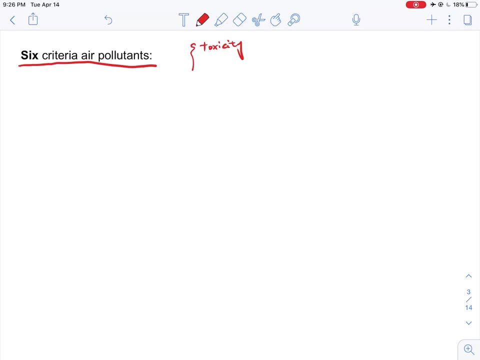 then we're less likely to categorize them as air pollutants, right? So on one hand, it's because of their toxicity, but also it's because of their quantity. So by meaning quantity, I mean these air pollutants are basically emitting in large quantities in the world, right? 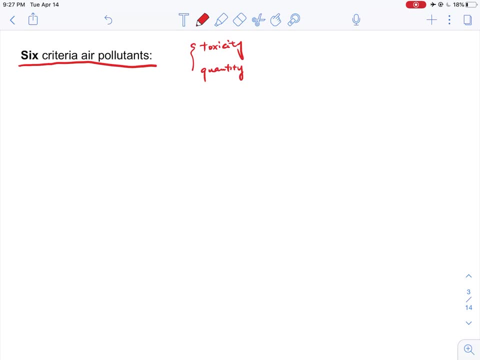 It's actually a combination of its toxicity and quantity that make them qualify as six criteria- air pollutants. So what do they include? So, for these six air pollutants, they actually include particulate matter, So we can also call them as PM, right? 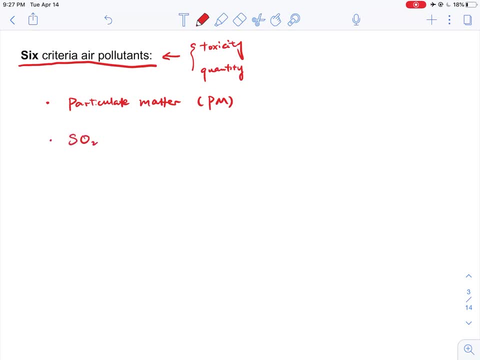 For short. So they also include sulfur dioxide, nitrogen dioxide, carbon monoxide, lead and ozone. Okay, So these different types of species are going to harm our health and also the environment in different ways. So let's just briefly introduce these six criteria: air pollutants. 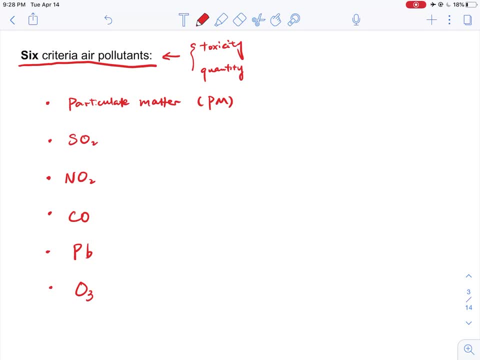 One by one. okay, So in terms of the PM, we don't like them. So basically, the PM are the dust or the suspended particles in the atmosphere, right? So, if you recall, we mentioned about suspended solids in the liquid right. 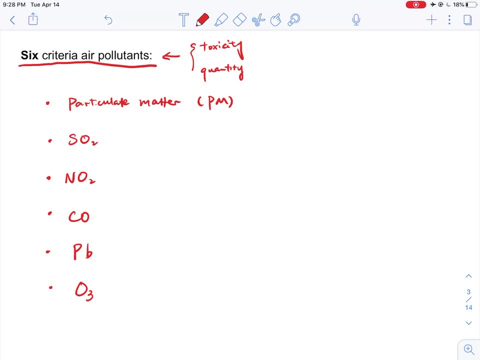 We also call them as colloids. So it's same as the particulate matter in the air, except that the medium is different. So we were talking about liquid in our earlier chapters and now here we're talking about the air. So these particles can also suspend in the air, right? 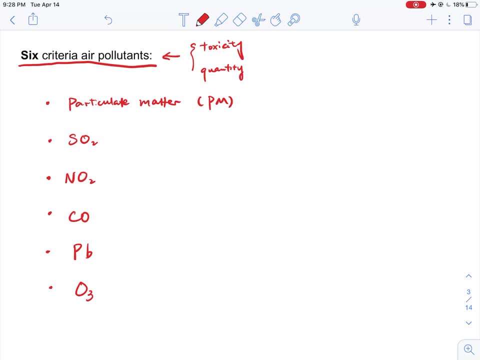 So they're toxic or they're harmful to our health, mainly because once we breathe them in, it's going to harm our respiratory system, So they may cause allergies or asthma, so on and so forth. Okay, And also we know that the suspended particles can affect our visibility, right. 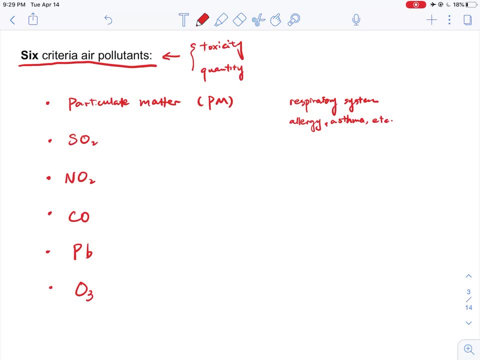 So sometimes if you go outside, let's say for outdoor activities, we see those air quality is not good, right, There are a lot of hazy or smoky environment in there, So it's also going to harm our mood in exercising right. 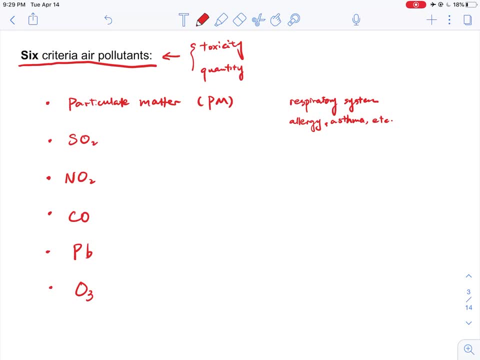 So that's why we can also call the PM as the air pollutant. So sulfur dioxide is also a criteria air pollutant. On one hand, it's because these sulfur dioxide can also get inhaled by human and then cause respiratory diseases. 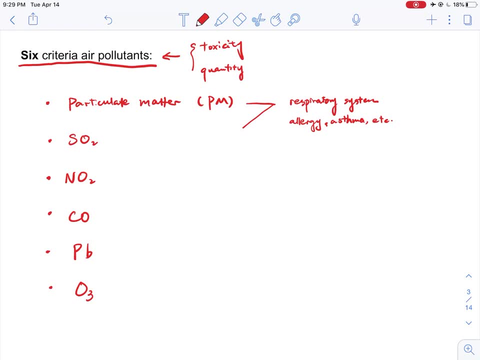 Basically they are also able to cause these allergies or asthma. But at the same time, as I have introduced earlier, sulfur dioxide can react with water right To form sulfuric acid. So basically we also need oxygen to further oxidize these sulfur dioxide to form the acid right. 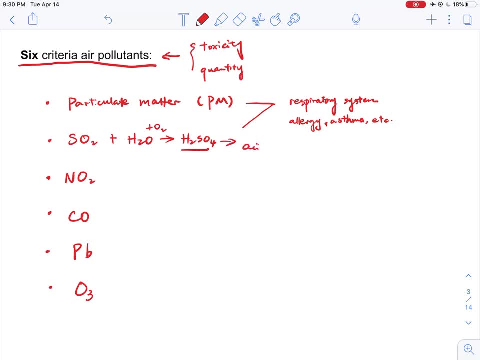 And then they will basically further form the acid rain, And the acid rain is going to damage the properties and also the plant life or animal life, so on and so forth. Okay, So you can see that the sulfur dioxide can actually pose hazards on two aspects. 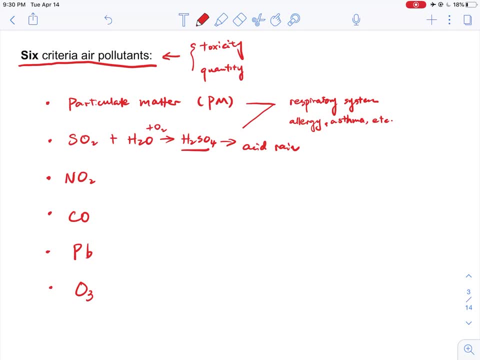 One is on the human health, the other is on the acid rain formation. Okay, So for nitrogen dioxide it's actually similar to the sulfur dioxide, So all the things can also happen for the nitrogen dioxide to our respiratory system, But at the same time they're also able to form acid rain, basically to form nitrogen or HNO3,. 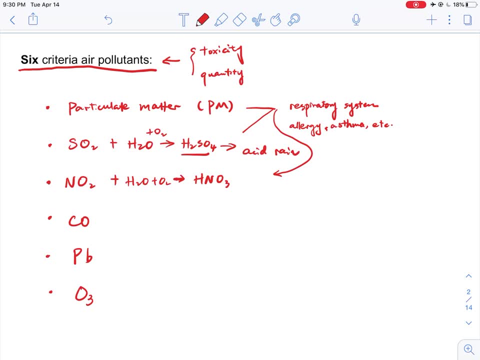 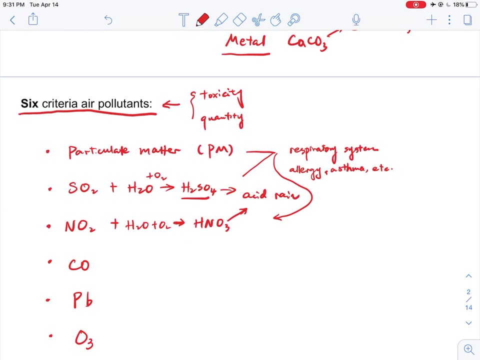 which is an acid right, A nitric acid. So basically they can also form the acid rain and further damage the properties. So you may notice that we were talking about NOx and SOx earlier, but here we were talking about sulfur dioxide or nitrogen dioxide. 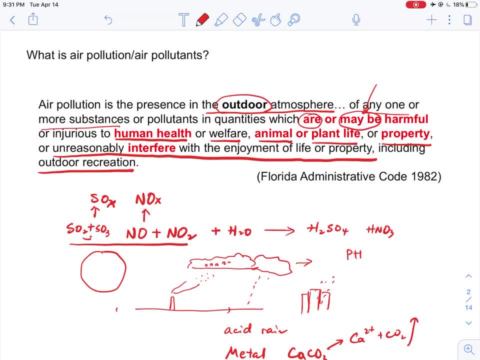 And this is mainly because, for different types of these oxides, they can really convert from one to another based on the temperature or relative humidity or pressure, so on and so forth. So there is a way for us to directly measure the SOx concentration, right. 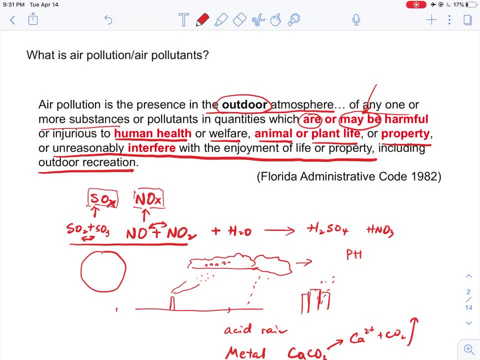 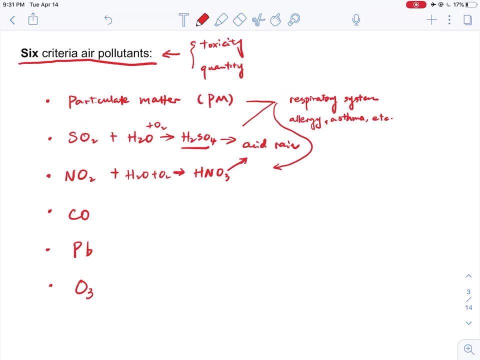 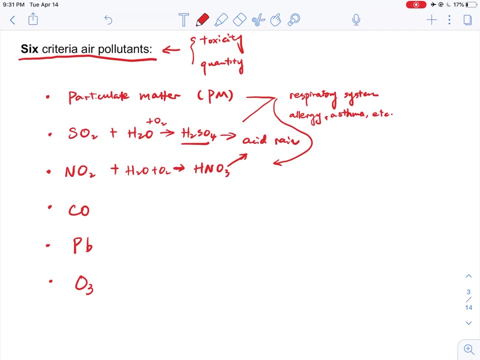 So, in terms of regulating these sulfur oxides or nitrogen oxides, people have to design or people have to define a specific type of the oxides. here And here, people just chose the most common form of these oxides. For example, for the SOx, sulfur dioxide is more stable, right? 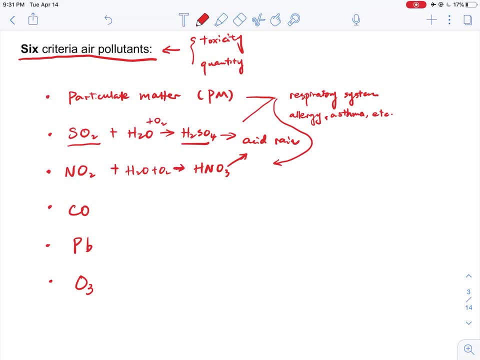 It represents a higher proportion in the atmosphere. So that's why we use sulfur dioxide as the form of this criteria- air pollutants- And similarly for the NOx, we're going to use nitrogen dioxide, Because it's more stable in the atmosphere. okay. 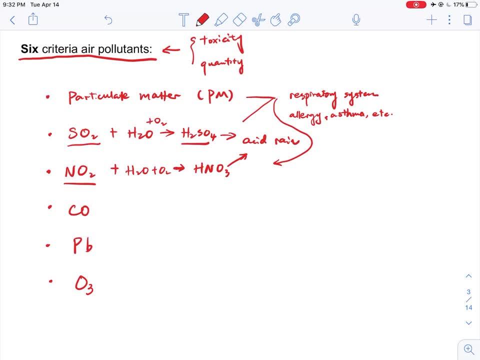 And further we have the carbon monoxide. So carbon monoxide is actually quite different from the previous three. It's mainly because the carbon monoxide can react with our red blood cell. So sometimes you may hear, basically from the early news, maybe 50 years ago. 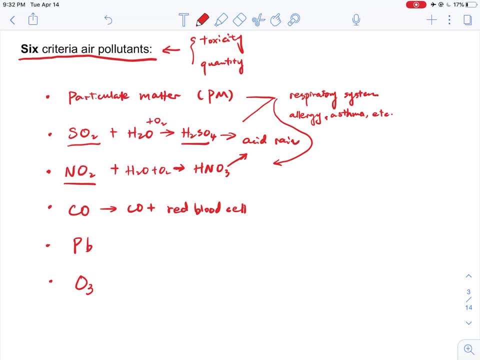 sometimes you may hear that people got dead because they breathe in or inhale too much of carbon monoxide. That's mainly because the carbon monoxide can replace the oxygen that's attached down to the red blood cell, Because we know that the red blood cell 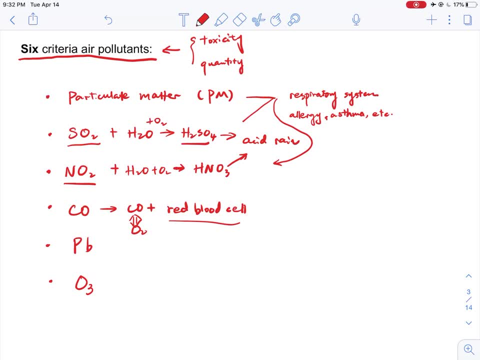 they're the carriers for the oxygen into our body, right, So they can be transported into the brain, to the heart, to all different muscles. But if there is a higher concentration of the carbon monoxide, so they will basically take the spot on these red blood cell right. 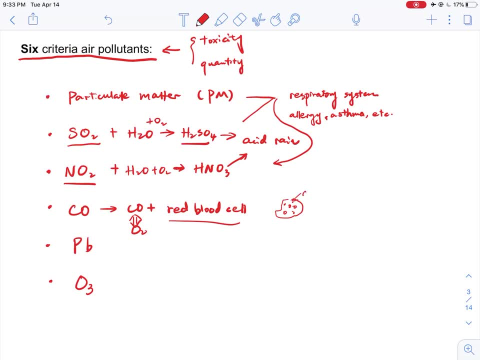 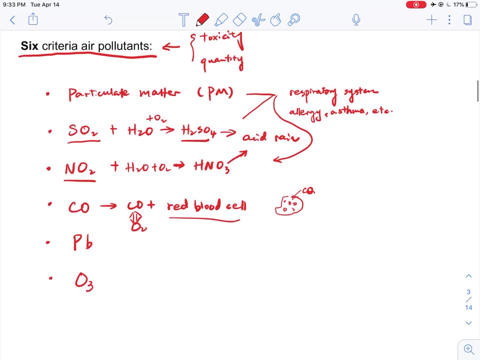 To replace them by carbon monoxide. So instead of sending oxygen into our cells, these red blood cells will send carbon monoxide instead. So in that case we're not able to oxidize all of the organics or nutrients in our body. 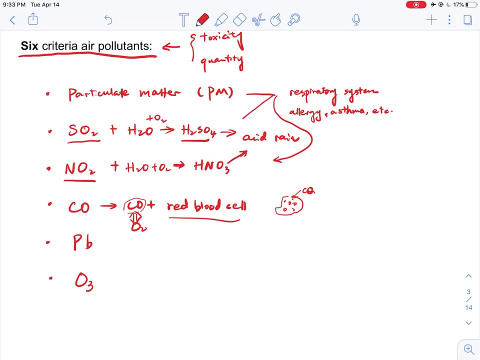 And then soon the cells will be dead. okay, So basically the carbon monoxide is going to react or cause the human health problems in a different way. okay, So lead is also one type of. the criteria are pollutant, So the lead is also one type of the heavy metal. okay, 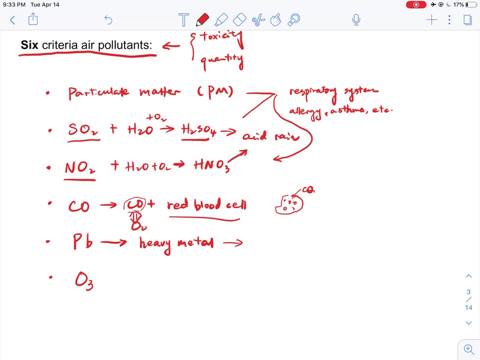 So the reason why we are interested or we take a lot of attention, pay a lot of attention to the lead is also because they can get accumulated in our body and specifically they can accumulate in our brain or liver and our kidney, And this is especially the case for young children because they're still developing. 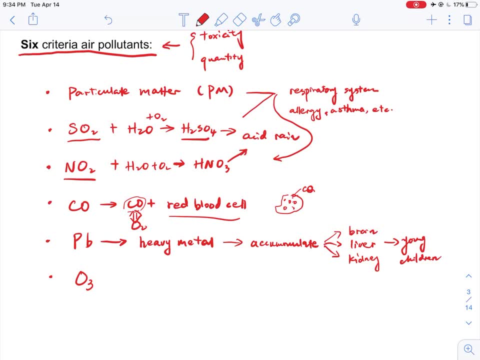 So all the cells are going to transport these heavy metal into these organs, right? Okay? So there are going to be more accumulation in these organs and it's going to seriously affect the health of the human there, specifically for the young children. okay, 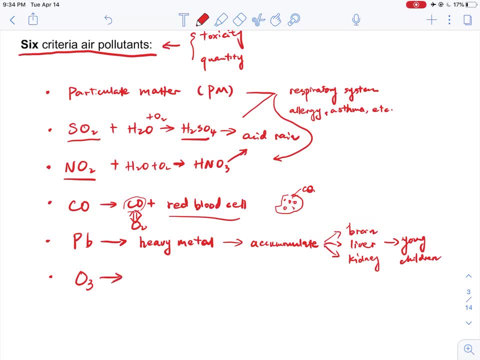 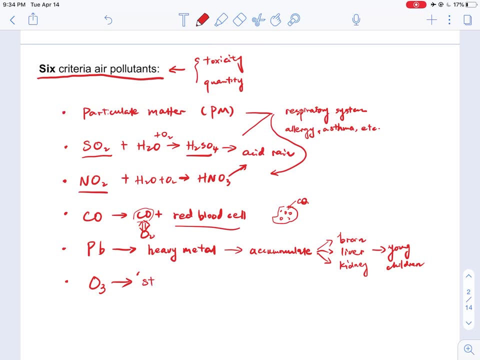 And further. finally, we have the ozone. So the reason why we also pay attention to ozone is because it's a strong oxidizing agent. So basically, they can oxidize a lot of things in our daily life, For example, for the tires, right. 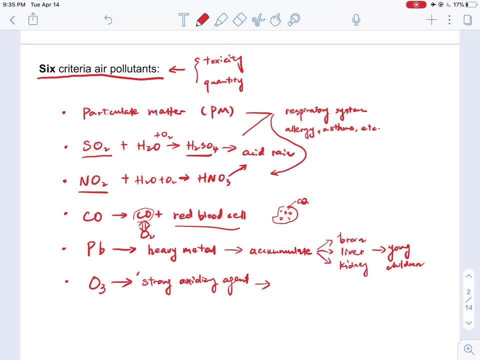 So if we leave those organics or polymers in the outside and we have a high ozone concentration, then those objects are going to soon get oxidized And at the same time, similarly to the particulate sulfur oxides or nitrogen oxides. 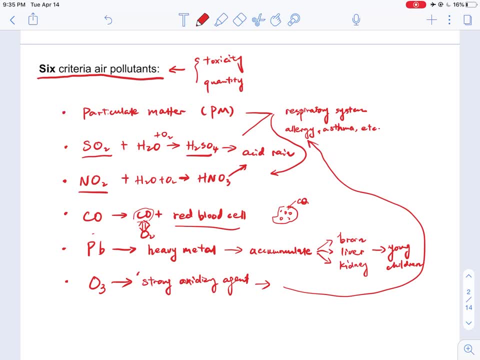 they can also cause the respiratory system to be damaged there. So on one hand, it basically damages the properties And on the other hand, they will damage our human health. okay, So, as I said, these six types of the air pollutants are most important. 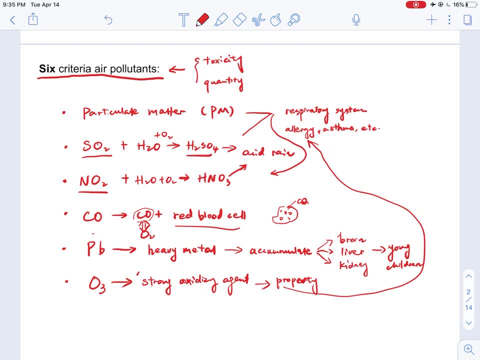 or we call them as criteria air pollutants, not only because they're toxic, right? Actually, they may not be the most toxic species in the atmosphere, because there can be other species, for example, like radioactive materials. We know that those are very toxic for human beings, right. 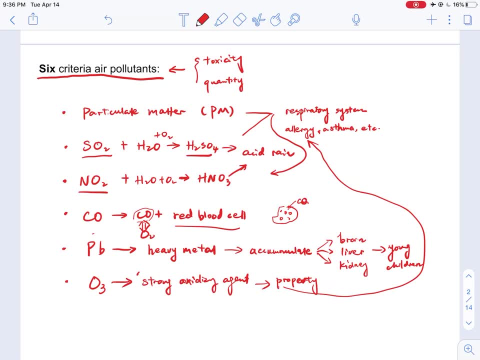 But in terms of the quantity radioactive materials are far less than the concentrations of these air pollutants right. So they can be commonly generated from a lot of daily activities. For example, for the particulate matter, sulfur oxides, nitrogen oxides. 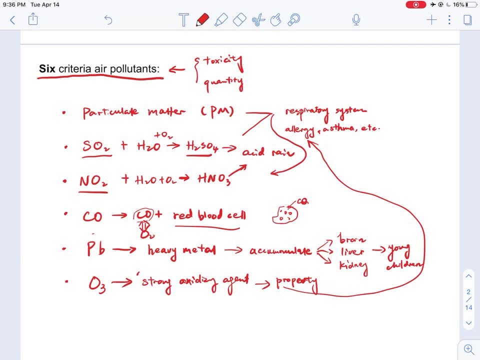 actually all of these can be generated from fossil fuel combustion, For example, the hydrogen oxide, coal-fired power plant or the diesel engine right car engines, because we do a lot of these combustion process and the combustion generate almost all types of these criteria pollutants. 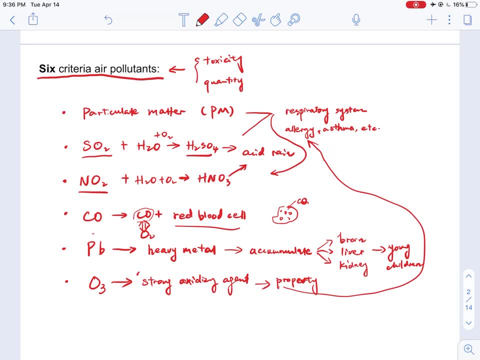 so we're. so it's because both of its toxicity and their quantity that we categorize them as criteria air pollutants. and further we can divide these criteria air pollutants into two types. so for the first five we can call them as primary air pollutants. okay, so by meaning primary air, 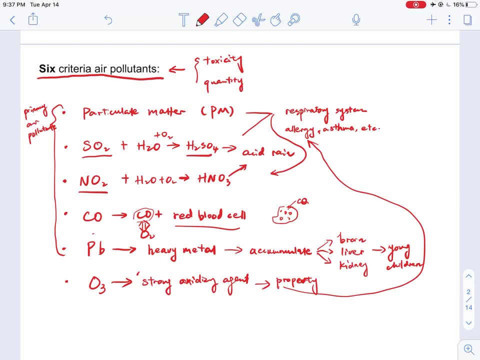 pollutants is not saying that they are further more important. it's just saying that they can directly get emitted from the sources. so it's direct emission, so they can directly come from combustion. and well, for the ozone here it's actually categorized as secondary air pollutant. okay, mainly because the ozone formation is actually coming from the indirect formation. 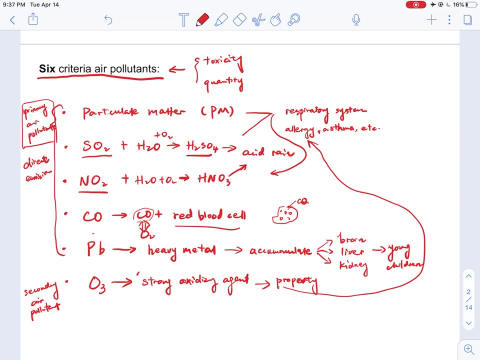 of existing air pollutants in the atmosphere. so if we talk about the combustion process, ozone is not directly coming from the flame. it's actually then the other pollutants, for example the nox and the voc, or the volatile organic compounds existing in the atmosphere, so they can further get oxidized by the photon that's coming from. 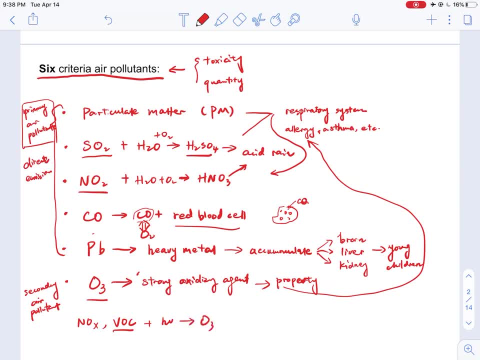 the sunlight or under the radiation, they will form ozone in the atmosphere. so the secondary air pollutants have to be formed based on existing chemical reactions. so we can. they are not directly generated from the um chemical reactions there. okay, so basically, if we go further into the details, so in terms of the ozone formation mechanism, 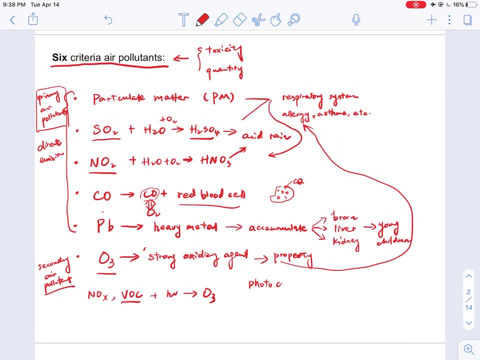 it is actually coming from the photochemical reactions. okay, so we have nitrogen dioxide, can further react and can first react with the radiation, and they are going to get split, split into an oxygen and nitrogen monoxide, and then this oxygen, or this oxygen radical, can further react with the oxygen to form ozone. 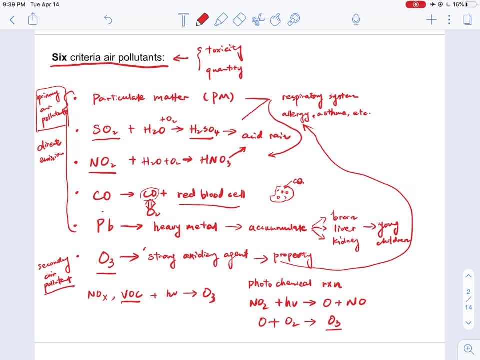 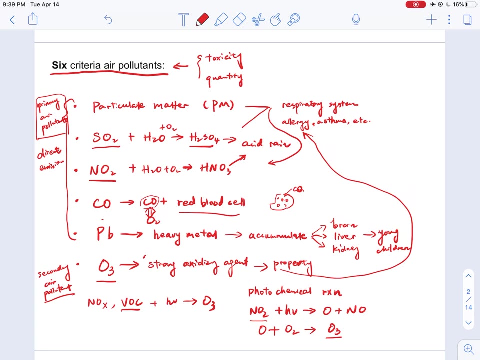 okay, so this ozone here basically is the indirect formation coming from the existing nitrogen dioxides in the atmosphere. so that's why we call them, call the ozone, as the secondary air pollutants. so just to reveal here for these six types of criteria, octetio per pollutants, we say: 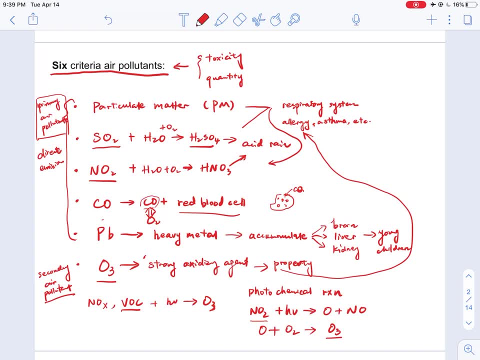 they're important because not only it's based on their um toxicity, but also is based on their quantity emitted into the atmosphere. and you can see it that a lot of them are harmful because they can cause respiratory diseases, basically cause allergy asthma, so on, so forth. right, so we can further categorize the first five of them as primary. 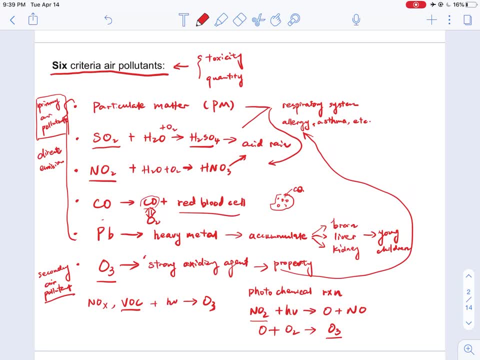 air pollutant because they can directly get emitted from uh chemical reactions, for example the combustion of the fossil fuel. well, for the last type of the air pollutant, or the ozone, we call it as a secondary air pollutant, mainly because it's not emitted, emitted directly from. 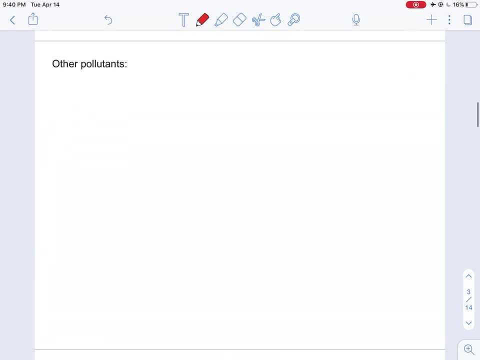 the reactions. okay, so, um, as i've introduced earlier, based on the definition of the air pollutant, there must be all different types of air pollutants, right? so here we'll just briefly introduce some representative air pollutants that are also quite important. so a major type of the air pollutant that are not categorized as the criteria. 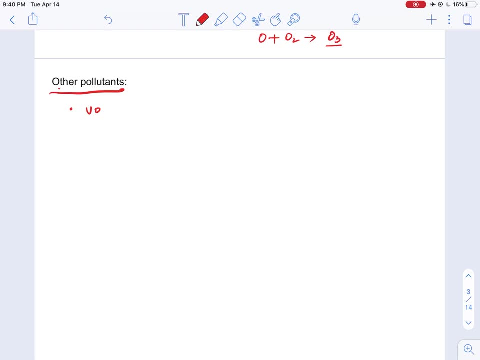 air pollutant, but also is quite important, is the volatile organic compounds or the vocs okay. so volatile organic compounds can include quite many different types of the gas species, for example the formaldehyde right, so formaldehyde has a chemical formula of h um ch2o right. so the formaldehyde mainly exists in new furnitures. 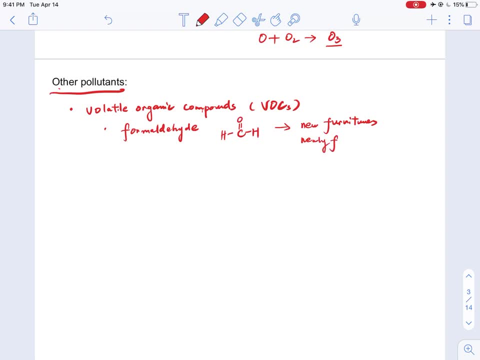 or newly furbished homes. 京a, cuscico, do you see q and ok this um? so this is ok. it looks so. the respiratory system, but in all the other parts of the body. So another example for the VOC is a benzene. 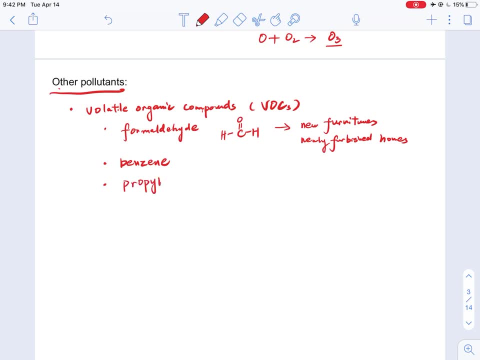 So there can be propylene, so on and so forth. So basically, all of these organic chemicals which are volatile in the atmosphere, we can categorize them as VOCs, So they're not only harmful to our human health, but also they're combustibles, right. 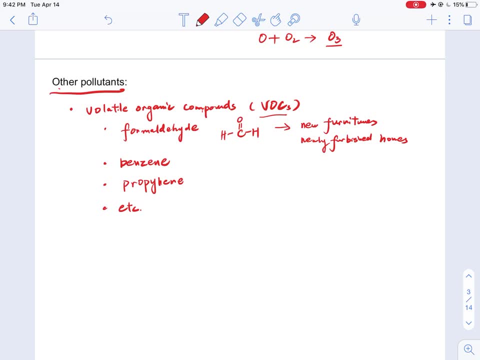 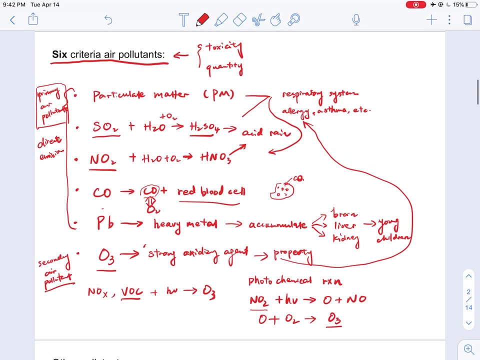 If we have enough of concentration in the atmosphere. they are also fire hazards, So there is enough reason for us to characterize them as air pollutants. But you can see that the reason why we cannot choose a single type of the VOC as the criteria- air pollutant- is mainly because there are just so many types of VOCs in the atmosphere. 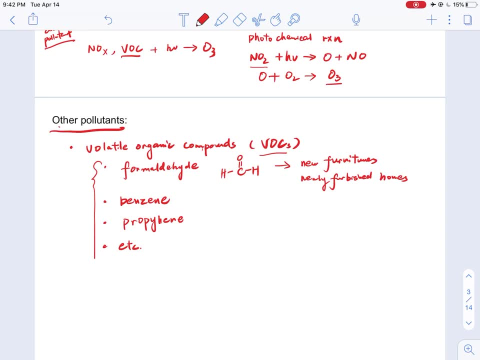 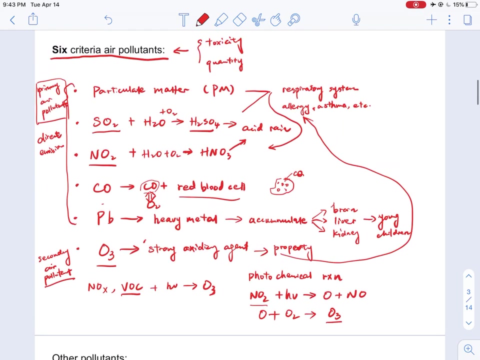 right And a lot of time. they can interact with each other, convert from one to another, right? So it's very difficult for us to track the concentration of specific VOC there, right? So, although maybe the total amount of the VOC that's emitted into the atmosphere might, 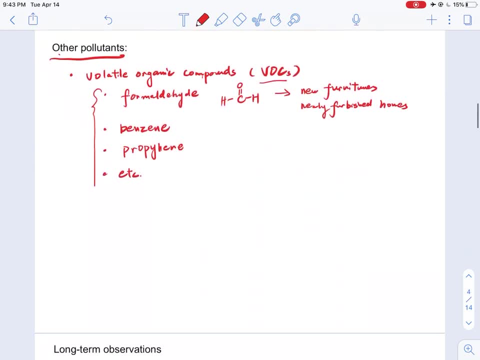 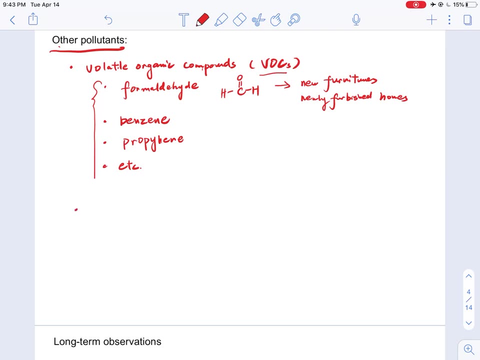 be comparable to some of these air pollutants, but the VOC here is just too complex for us to track all of them right. And in terms of other pollutants we have introduced that lead is one type of air pollutant right. It's a type of the heavy metal right. 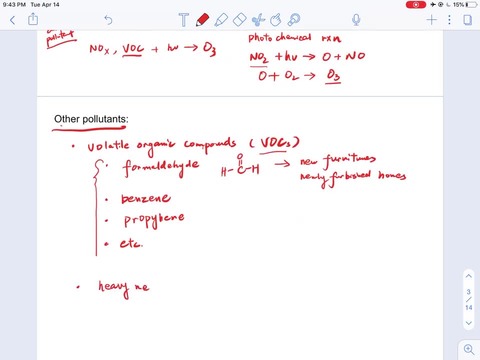 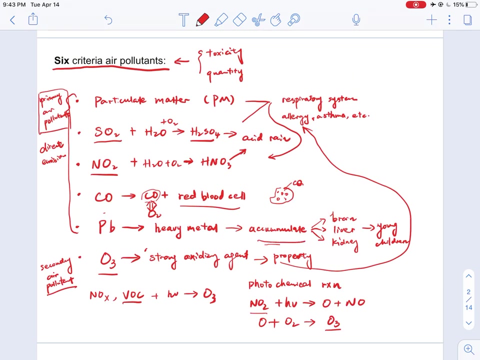 So there are also other heavy metals, for example, arsenic right, And also mercury, so on. okay, So basically the common feature for all of these heavy metals is that they can get accumulated into organs, right Different types of organs. 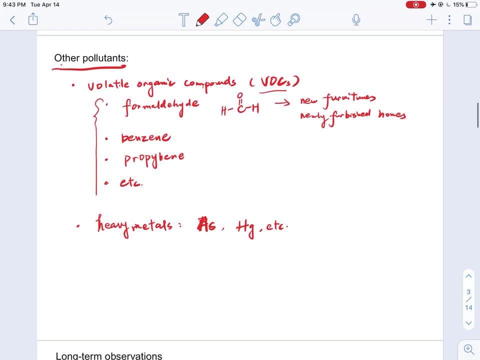 It's just lead- are emitted with a higher quantity. It's a higher quantity into the atmosphere, right? So we also mentioned that radioactive materials. So radioactive materials are also representative types of the air pollutants. So you can see that there are all different types of air pollutants here. 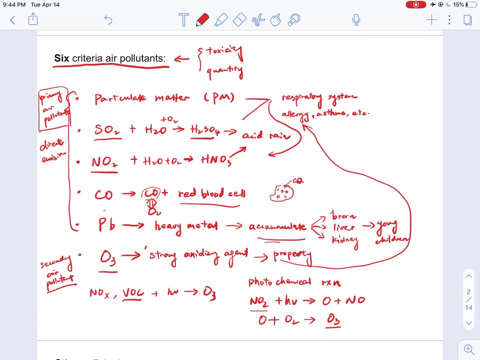 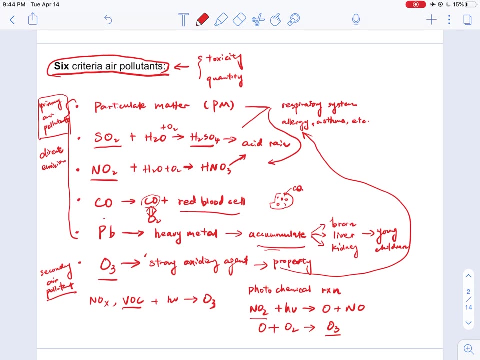 But for simplicity in terms of the air quality control, we will just study this. Okay, Thank you. We will just quantify or constrain the emission of these six types of the air pollutants. okay, So in this class we're just going to go over the emission or the sources of these criteria. 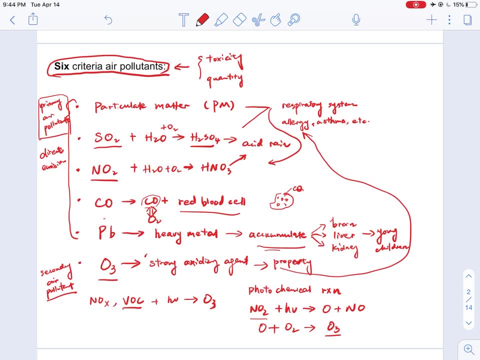 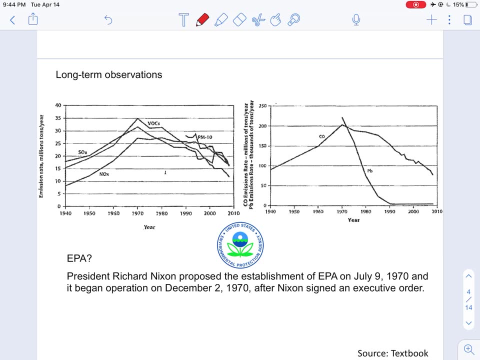 air pollutants and also the control methods of these air pollutants. So here I'm also showing a long-term observation of the emission amount for these six different types of criteria air pollutants. So you can see that I labeled. here we have SOX, NOX, right, VOCs. 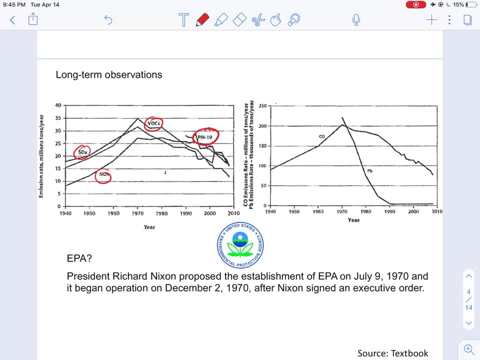 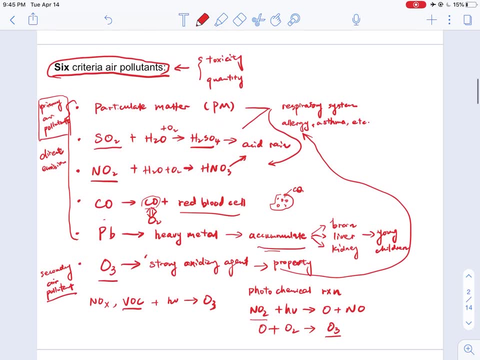 So VOC, again, is not a type of the criteria. air pollutants: We have PM10, right? So you may wonder what does this 10 represent? So PM- we mentioned that it's particularly matter, right? So PM10 simply means that the particular matter that are below 10 micrometer. 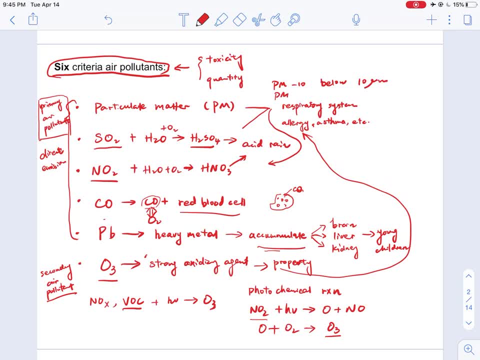 Okay, Thank you. So we probably also have heard of PM2.5.. So, similarly for PM2.5, they just mean the particular matter that are below 2.5 micrometers. So we'll further introduce why we're basically separating them based on their sizes. 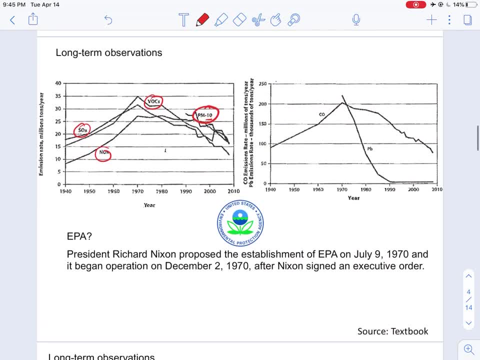 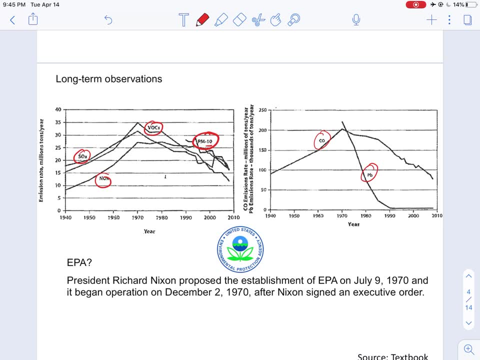 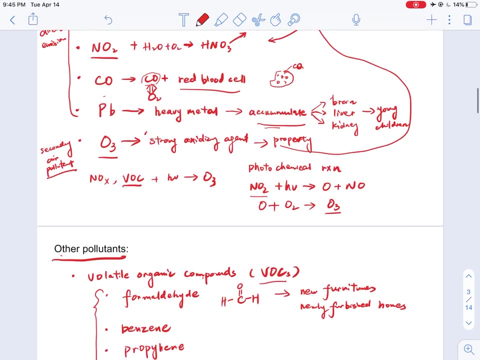 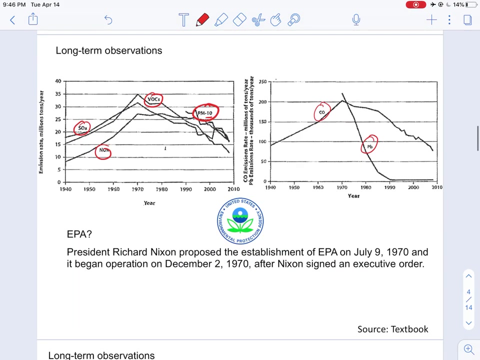 It has something to do with our human health here. okay, So here is also listing the emission amount of the carbon monoxide and lead, right? So if you quickly check here, there's one criteria- air pollutant- missing, right? So we didn't show the ozone here. 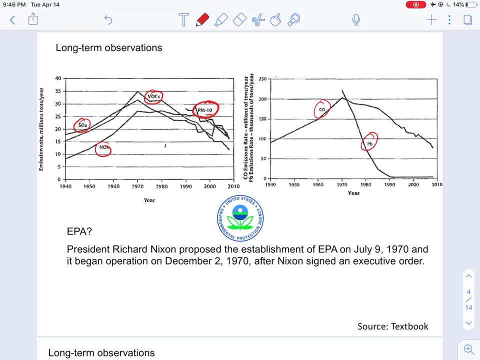 So on one hand, it's because the ozone, so it is mainly. actually. it's mainly because ozone is not a primary air pollutant, right, It's not directly emitted into the atmosphere, We can only measure the concentration, right. 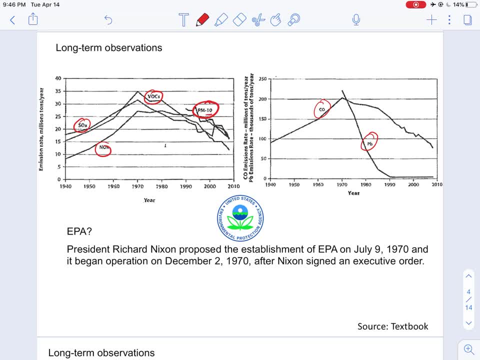 But it's not coming from a direct source. Okay, It's coming from a source or from the chemical reactions, But here we're monitoring the emission amount right. So this is directly coming from the emission sources. So therefore, we're just limiting, we're just showing the emission rate of these primary 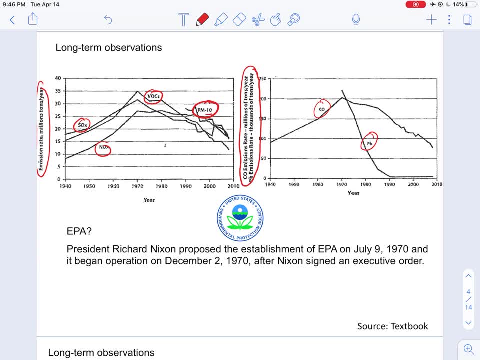 criteria: air pollutants. So by tracking these trends you can actually notice a great feature or common feature in all of these emission amounts, right, So you can see that. Okay, So in the year of 1970, it seems that all of these air pollutant concentrations, or their 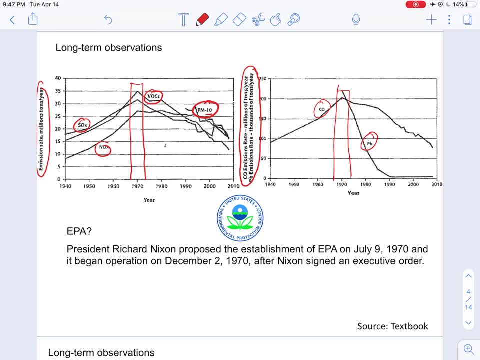 emission amount decreased right, So we reached a peak point here and then the emission just went down. So we know that a lot of these air pollutants are related with fossil fuel combustion And actually statistics show that. Okay, Okay, Okay. 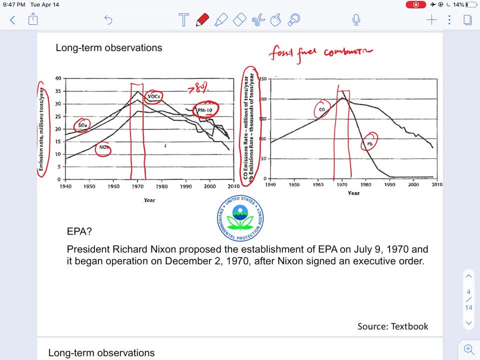 So we can see that about 80%, actually more than 80%, of the particulate matter are coming from the fossil fuel combustion. Well, almost all of the nitrogen oxides, nitrogen or NOx, are coming from the fossil fuel combustion. Okay, 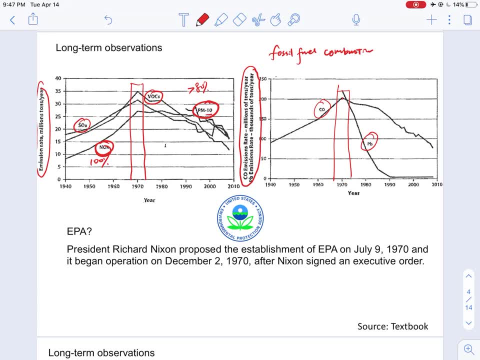 So why do we burn fossil fuels? It's because our economy needs that right. We need to drive cars, We need electricity, We need all of different forms of the energy to drive our economy, But what we're noticing is that Okay. Okay, So in the year of around 1970, all of these emission amounts decreased. So why is it All? right, We didn't have a Great Depression during this period of time? right, It is actually because of the establishment of the EPA. 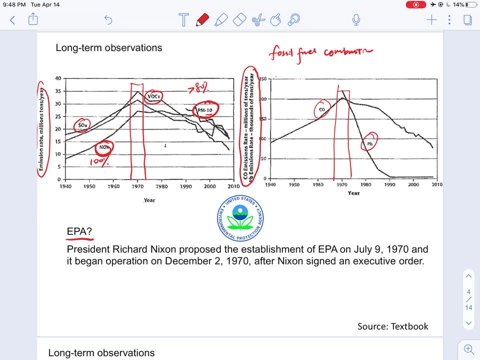 So the EPA is short for Environmental Protection Agency, right, This is the agency that has the right or has the authority to enact different types of policy and then to control the quality in different mediums, right? For example, the air quality, water quality, soil quality, so on and so forth. So, basically, in the year of 1970,. President, Richard Nixon proposed the establishment of the EPA on July 9th 1970, and it began operation on December 2nd 1970. So, basically, the EPA started in 1970, and you can clearly see this drastic change in the emission of these primary air pollutants. right, So you can see that the 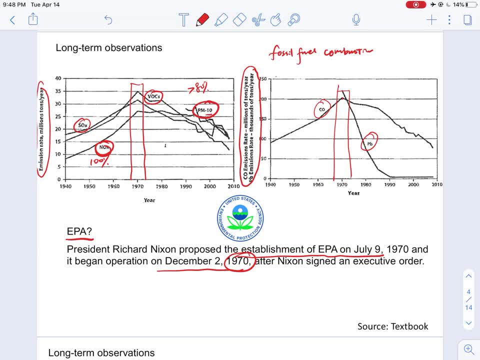 policy really can work in terms of controlling the air quality there. So it also applies for other types of, for example, the water quality, soil quality and so on. okay, So that's why we want to learn how important or what is the mechanism for the emission and for the control. 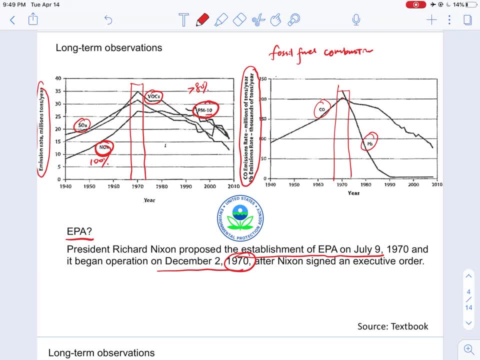 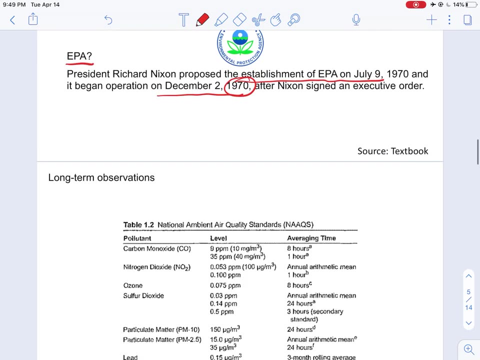 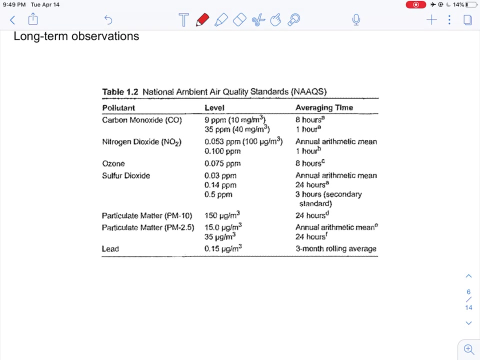 of these air pollutants, so that we can inform these stakeholders or policymakers, so that we can enact the policies that can reduce the air pollutants, reduce the water pollutants, while protecting our economy right? So, basically, the EPA also enacted the requirements in terms of the air quality standards. 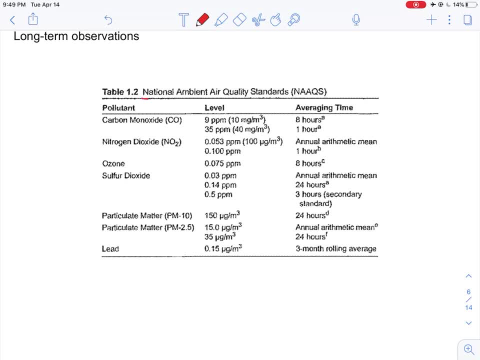 So we have an air quality standard that's called the National Ambient Air Quality Standard, or the AQS. So this air quality standard regulates what are the required or the standards for the concentrations of these six criteria- air pollutants. So let's go over them again, right? We have carbon. 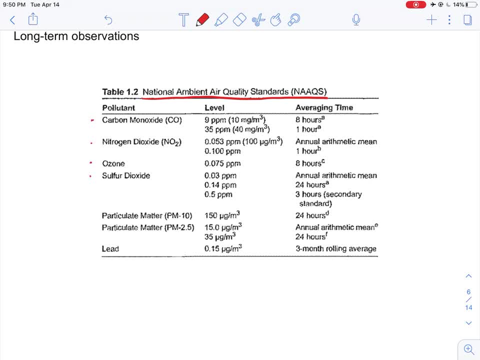 dioxide, nitrogen dioxide, right Ozone, sulfur dioxide, particulate matter. So notice here that we have PM10 and PM2.5, and we also have lead right. So there are six of them, So further you can see that, basically for different averaging time, for different monitoring time. 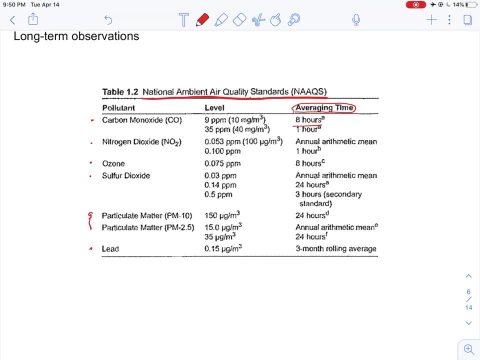 we have different standards, right? For eight hours, the carbon dioxide concentration, or the standard, is 9 ppm. ppm means parts per million, right? And if we're measuring just for one hour, then the standard is 35 ppm. So we mentioned from quite many times earlier that we use different. 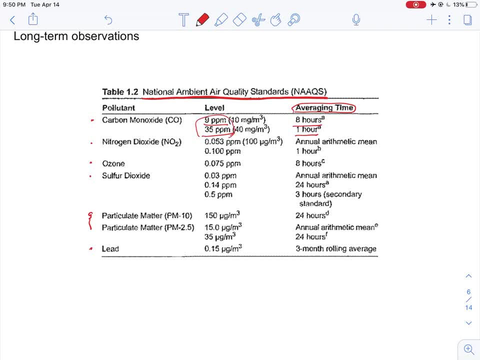 time or we use different standards. if we use different averaging time, mainly because there are fluctuations in terms of the concentrations for these pollutants, right, For example, if we're just monitoring for one hour during this time, then maybe accidentally there are some emission. 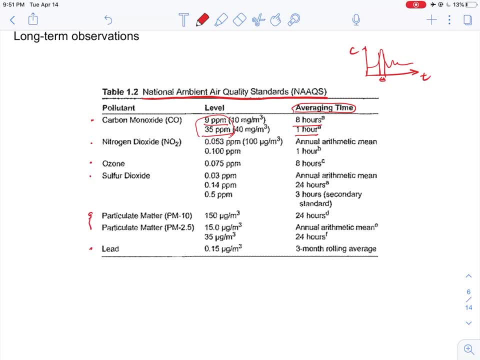 of these air pollutants. right Because of that, since we use a shorter monitoring time, so the standard can be higher. Well, if we monitor for a longer time, then the standard should be lower. right Because you're looking at a cumulative effect of all of these air pollutants in there. 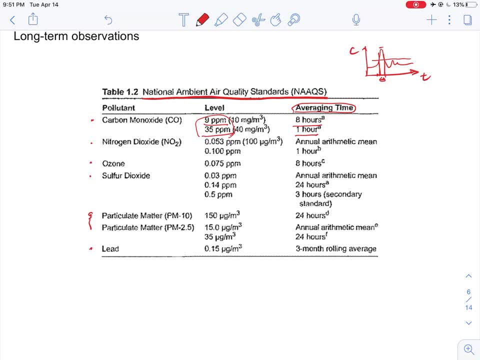 So from this table, you can also notice that we actually show different units here, which some of them showed PPM, right. You can also see that in the bracket we're showing a differentwith a different unit, which is 10 milligram per meter cube, right. 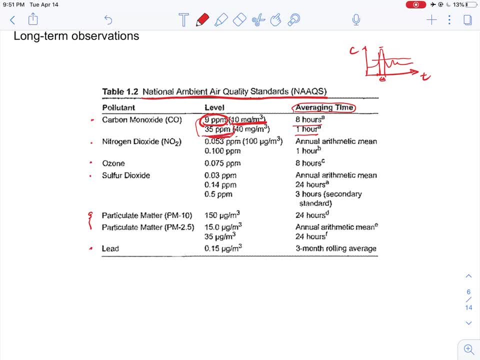 And, For example, for 35 ppm, we also have some value- that's around 40 mg per cubic meter, right. And similarly for the nitrogen dioxide. we also have these two different units, So are they equal to each other? So they should be right. Because if they're different from each other, then the industries they will just use whichever that has a lower value. This doesn't make sense, right? If we have a lower value with different unit, then why do we still establish another number there? 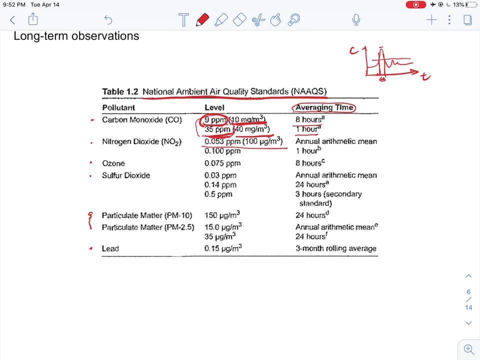 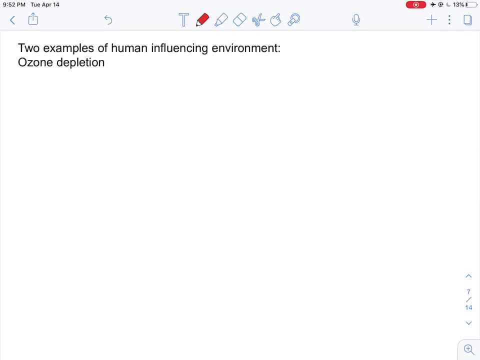 So they have to be equal to each other, right? So therefore we need to do some calculation to convert these different units, or different values, in different units there. So we'll probably do that at the end of this class here, okay? So here I'll guide you through two examples on how human might influence our environment, right? 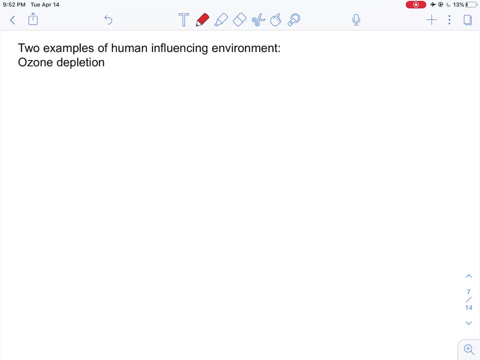 Because a lot of time we were saying that, well, human are just, we can just live by ourselves. right, We can just work on our economy, use our industry. There's no need to care about the planet, We just need to care about ourselves. 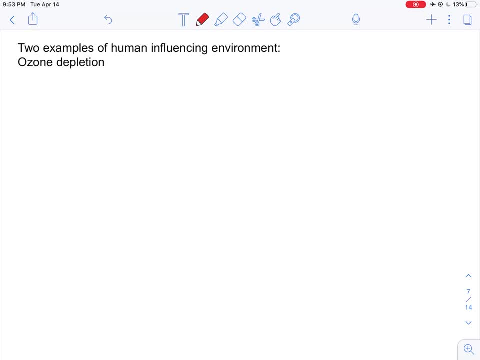 But that is actually quite selfish, And there's more evidence showing that we human beings are polluting our environment. It's causing global issues. So one example: What we're quite interested in is the ozone depletion. okay, So by looking at this name here, you may say that well, is ozone depletion a problem? 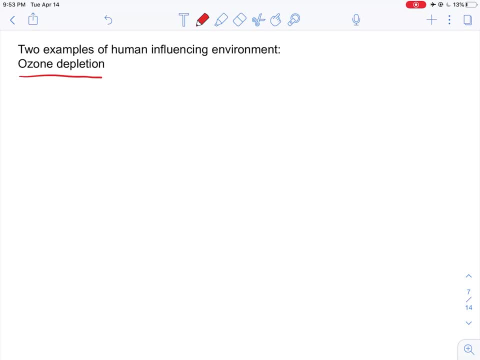 Because we just learned that the ozone is a criteria- air pollutant- right. It's not only an air pollutant, It's actually the most important air pollutant in the atmosphere. So the ozone depletion- why is it a problem? The more we deplete it, the better, right. 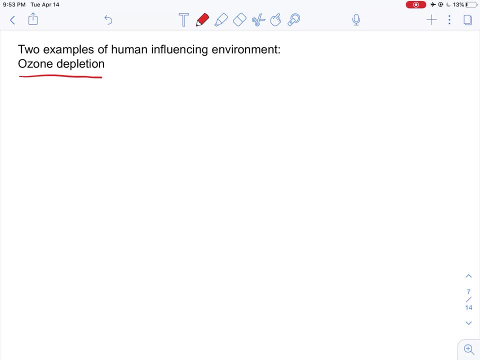 But actually it is not the case. It really depends on where the ozone is located. So, for example, let's say we draw our Earth here, okay, Let's also draw our continents right. We have Asia, right. We have North America, South America, right. 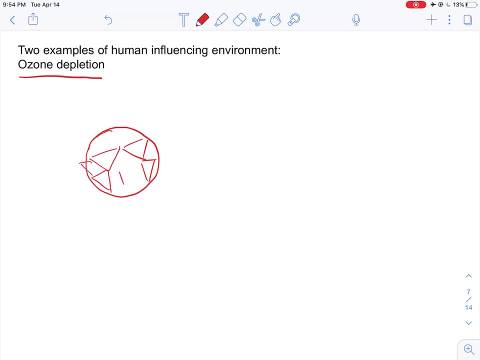 And then we have Africa and Europe, okay, And then we have Australia here, okay, And then the Antarctica. So this is our Earth, okay, And this actually looks pretty cool, right. So in terms of the atmosphere that we're talking about, so there's one layer of air that's surrounding our Earth. 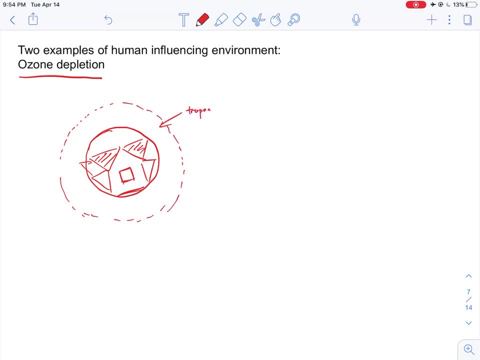 and this layer of air is called the troposphere. So the troposphere is typically within the range from five to 10 kilometers from the ground. okay, So if we are talking about the troposphere in the equator region, then this height is around 10 kilometers. 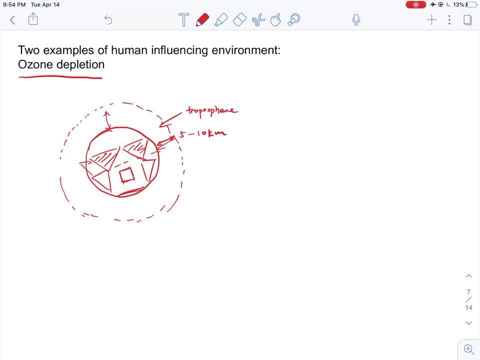 If we're talking about the height that's at the polar region, it is around five kilometers, right? So you can see that I would say almost all of the human beings live in the troposphere, right, Except for those astronauts that's living in the ISS International Space Station, right? 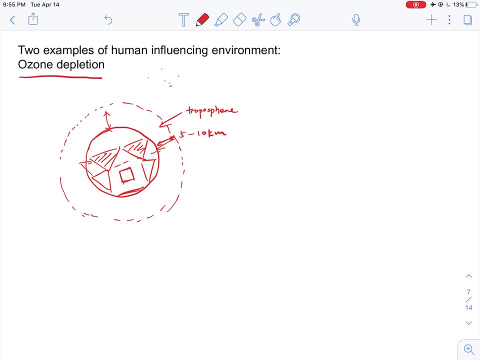 It's just, let's say, 10 or 20 of them. 10 or 20 of them, right, But most of the human beings are living in the troposphere. So if there's ozone in the troposphere, since the air makes so well in the troposphere- 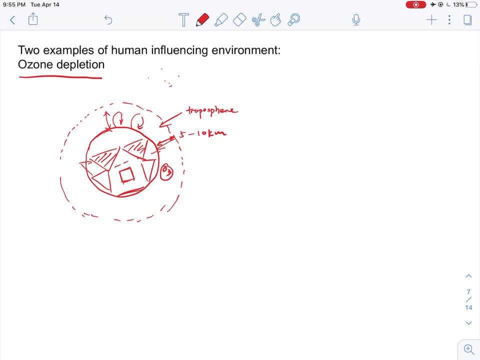 then the ozone here is going to be an air pollutant right. It's also a criteria air pollutant which is bad for the human being or for the human health there. So above the troposphere there's a layer called the stratosphere. 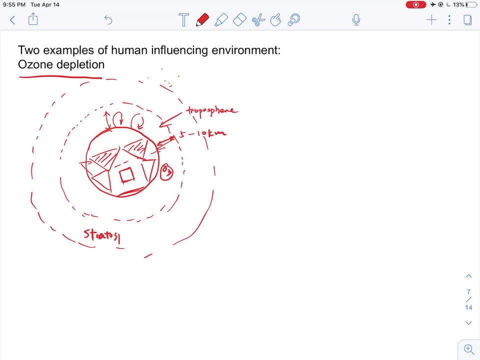 So inside the stratosphere there's a high concentration of ozone. So there's a high concentration of ozone. So actually this layer of ozone protects us from being directly bombarded by the radiation from the sun. The sun generates a lot of strong energy radiation. 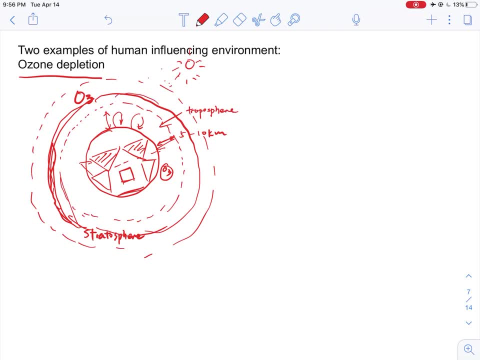 And the ozone layer actually helps us block the ultraviolet radiation, so protect us from the skin cancers, okay. So the chemical reaction that's happening is actually ozone can react with the radiation, right? Actually, it's also high-energy radiation, UV radiation, and we're going to generate oxygen, and oxygen radical. 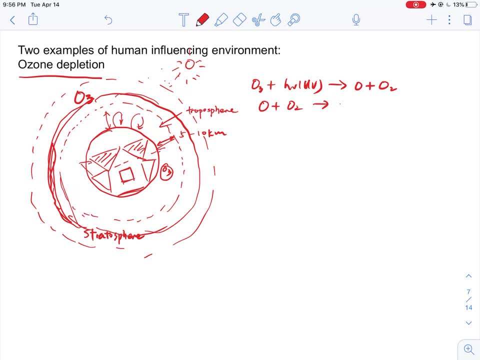 And further, the oxygen radical can combine with the oxygen and form back to ozone again. right, So yeah, You can see that basically what happens is that the ozone converts this radiation from the UV radiation, UV light, into heat. okay, 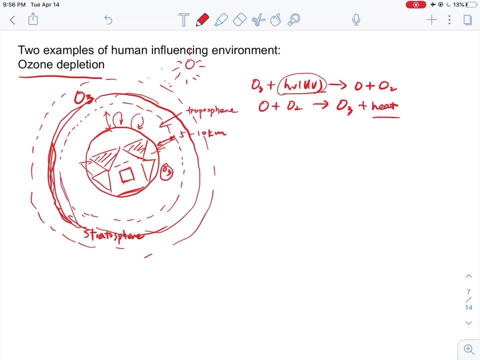 And in this way the ozone layer actually protected people from getting sick, right? And what happens is that, with the emission of a lot of chemicals from the human being, the ozone layer that's in the stratosphere is getting interfered, is getting depleted. So one thing I forgot to mention is that, because of the temperatures or structure of our atmosphere, there's no strong mixing between these two layers. You may wonder: why don't we just emit these ozone? Why don't these ozone just float up to the stratosphere? 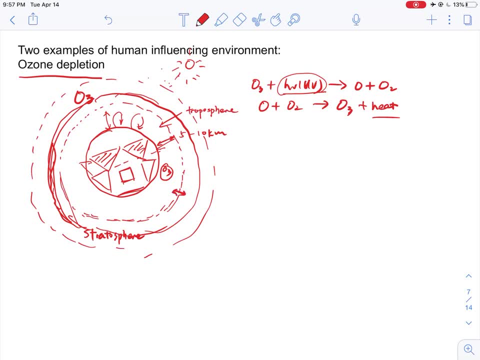 It's very unlikely, right. So there's maybe some small stream that's being transported. Some of them are being transported up to the stratosphere, But most of the air are constrained in the troposphere there. So that's why a high concentration of the ozone in the stratosphere doesn't necessarily mean a high concentration of the stratosphere. And also the ozone in the stratosphere is not very easy or very difficult to transport to the surface of the Earth. Okay, So then people? So, actually, it was until recently that people started to realize that the ozone concentration in the stratosphere is very, very high. 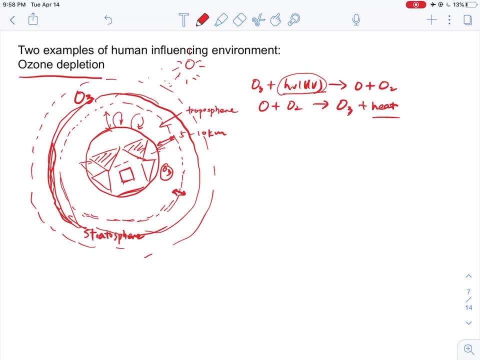 Okay, So then people? So, actually, it was until recently that people started to realize that the ozone concentration in the stratosphere is rapidly decreasing, And the reason for this ozone depletion is because of the chlorofluorocarbon, or the CFC. 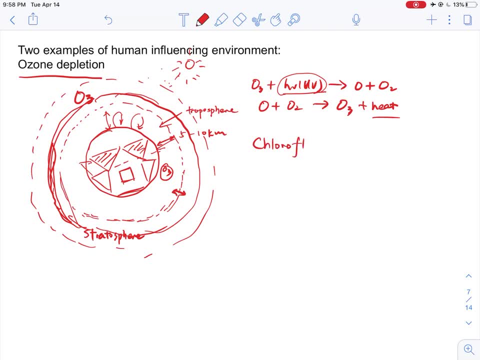 And the reason for this ozone depletion is because of the chlorofluorocarbon or the CFC, So for short we call them as CFC. Okay, So if you use a, So if you use a, If your family use a very old refrigerator, 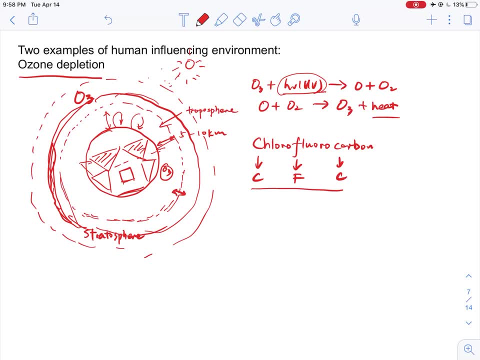 sometimes you may say you may notice that the refrigerator doesn't freeze really well. So then people will say that, oh, why don't we just fill in more liquid in there? So actually the liquid we use in the refrigerator is the CFC. 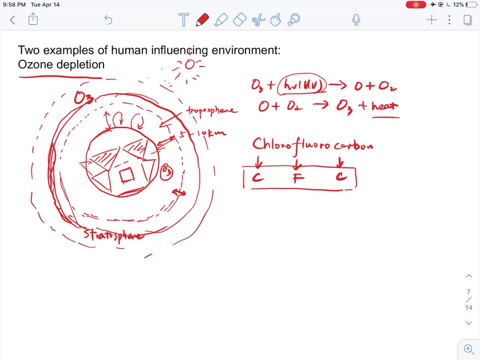 And this is the case for many old refrigerators. So what happens for the CFC is that the CFC When people first invented this chemical. so we need to also notice that this chemical is not natural. So people invented this chemical from the industrial plants, right? 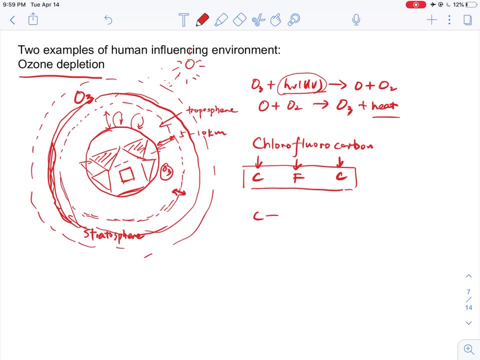 Because if you look at the structure of the CFC, it's mainly just carbon in the center, and then you have fluoride or chloride at the branch. So there's no way the environment or the nature can create something like this Right. It almost looks perfect in terms of its structure. 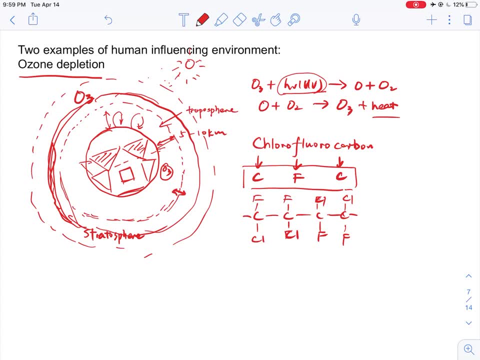 But the industrial plants? they can use some chemical reactions to generate these species. The reason why people like this chemical is because they're very stable. Okay, So people have been using- actually have been using- sulfur dioxide as the refrigerant for keeping things cool. 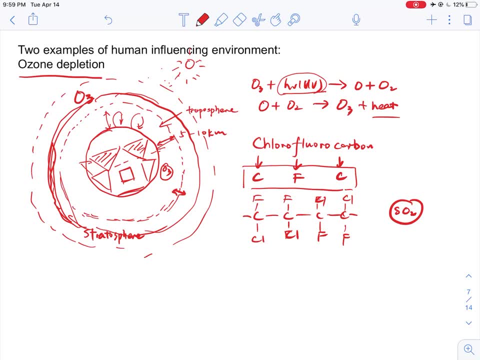 And you can think of the hazard that's associated with sulfur dioxide right. Once it gets leaked, it's going to emit a lot of these toxic gas into the atmosphere, Right, And people won't feel comfortable in smelling them. So people realize that the CFC is very stable. 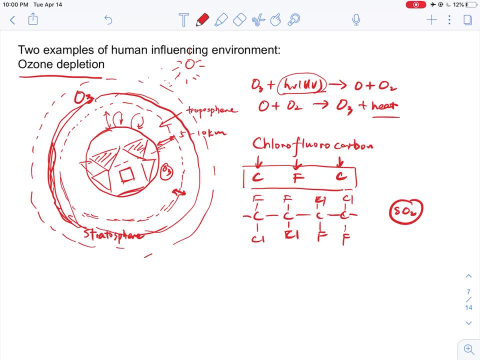 There's no way they can get harmful to the human being Right, Even if we breathe them in. since it's very stable, we can just directly exhale them out, But by being stable in the stratosphere for the CFC. 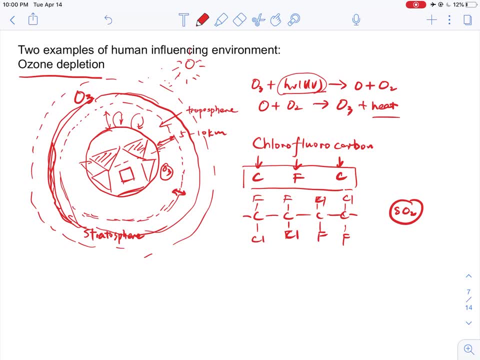 doesn't mean that they'll also be stable in the By being stable in the troposphere doesn't mean that they're stable in the stratosphere. So people realize that the CFC can also get reacted under UV radiation. So what happens is that 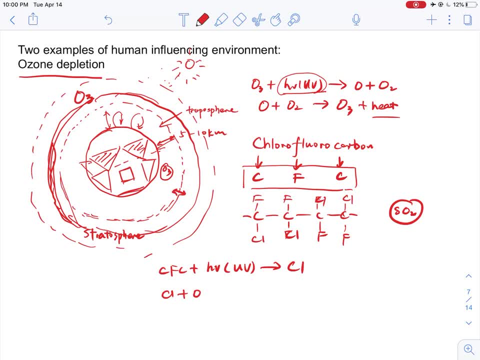 it's going to emit a chloride radical, And this chloride radical can react with the ozone almost endlessly- Okay. So if you look at what is happening in this equation here, Okay, The chloride radical can react with the ozone, form the oxygen and chloride oxide. 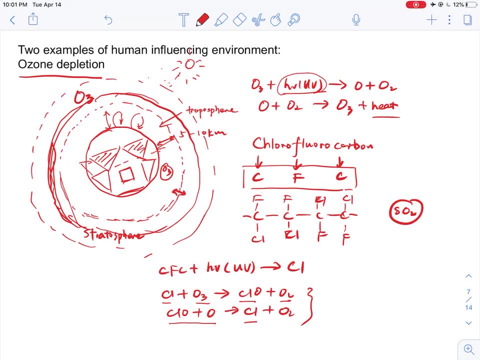 or the ClO- Right. So further they can react with the oxygen radical and form chloride back again. So you can see that by being reactant it also get converted back into Converted back again Right. So the chloride radical is not being consumed. 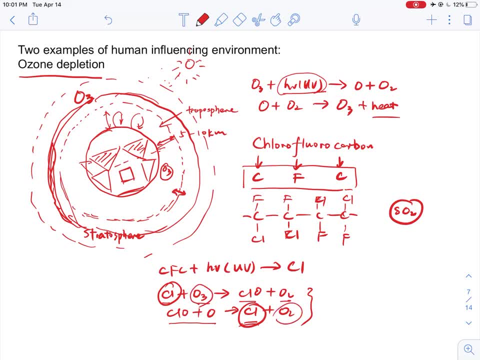 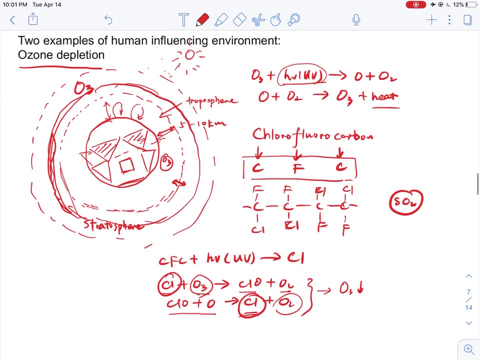 from this reaction here, While we're converting the ozone into oxide, Into oxygen. So basically, under the UV radiation, the ozone concentration will decrease Right. So this is especially the case for the polar region, Mainly because once we emit this CFC into the atmosphere, 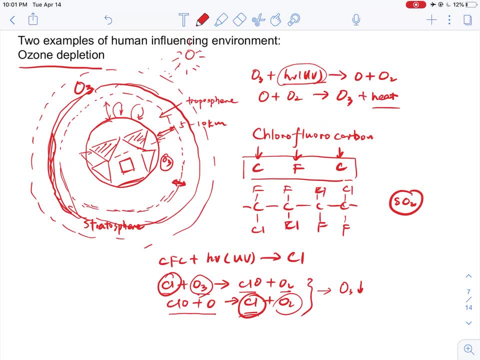 right, Although we said that there's limited transport, but once even one molecule get emitted into the stratosphere, they can just being stable there for endless amount of time. Right, Because there's no way we can destroy these chloride radicals, But the chloride radicals are constantly destroying. 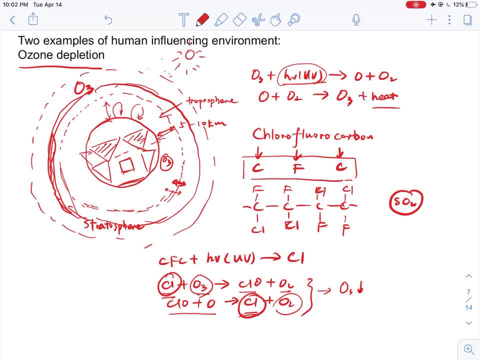 the ozone in the stratosphere And also once they get emitted into the stratosphere and further get leaked into, Once they get emitted into the troposphere and further get leaked into the stratosphere. the polar region is relatively more stable in terms of the air motion. 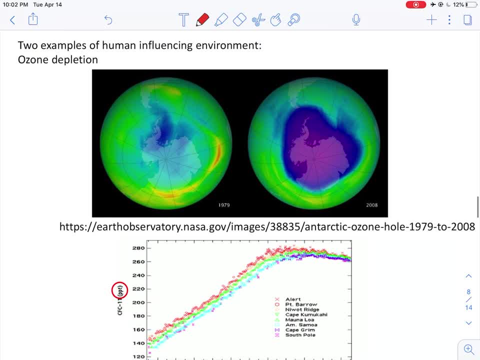 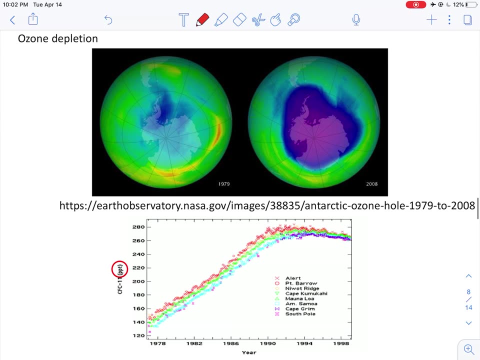 So that's why people can notice this enormously large ozone holes here Right, And this is specifically for the case for the Antarctica region. So actually people have been tracking the CFC concentration in the atmosphere And you can see that the concentration has been increasing all the time. 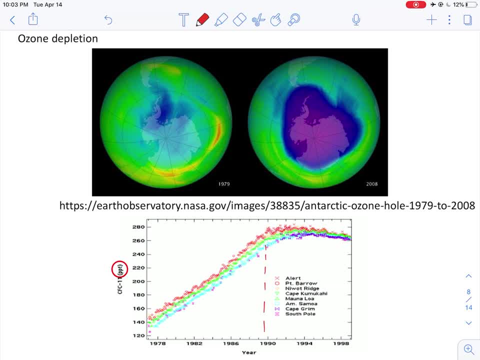 until around the year of 1990.. And this is actually because people started to realize this issue, or this is a very important issue, Right? Just think of, Think about the ozone depletion or the ozone hole here. So there are still a lot of animals. 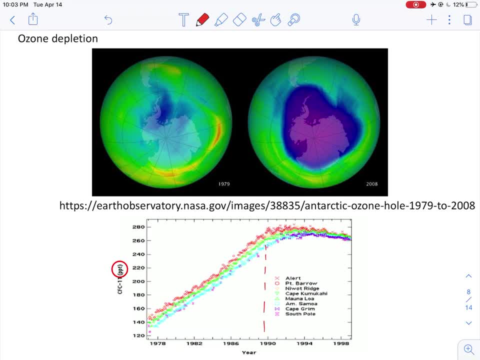 living on Antarctica Right By emitting the Or by forming this ozone hole, then the UV radiation can easily penetrate through the atmosphere and then cause skin cancers or all different types of diseases to the animals living there, And nowadays people are also observing. 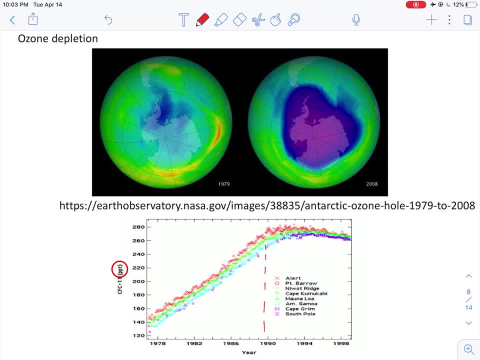 ozone hole in the North Pole And there are more European countries under the issue, under the influence of this issue here. Okay, So what happens nearby the year of 1990 is because people signed- Almost all the countries get together and signed the pact. 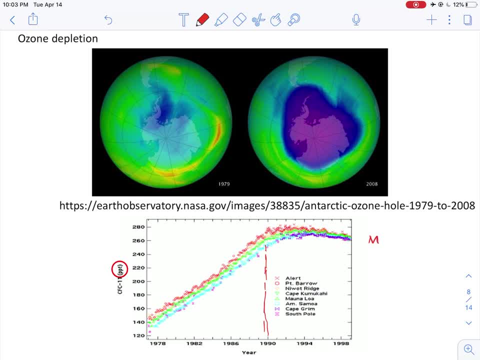 or signed the policy of the Montreal Protocol. So it was signed at 1989.. Okay, So you can see that immediately after this policy gets into the, Get into the daily life, or get into the industry, the concentration of the CFC started to halt. 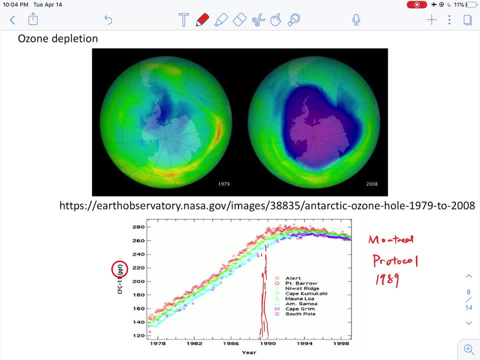 Right, It's not increasing anymore, But you can also see that the concentration actually decreased very slowly. This is because the CFC is very, very stable. There's no way we can destroy them in the atmosphere. Okay, So it's still. 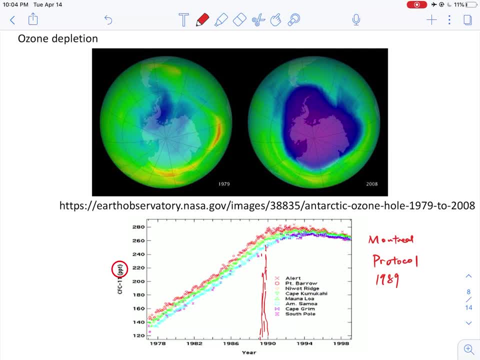 What that means, simply, is that the CFC is still getting leaked into the stratosphere and it's still actively reacting with the ozone in the stratosphere. So from the news you can see that the ozone hole is actually expanding year after year. 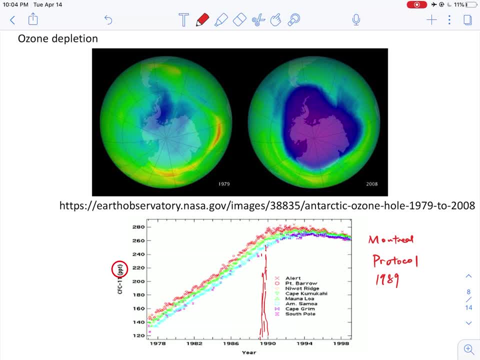 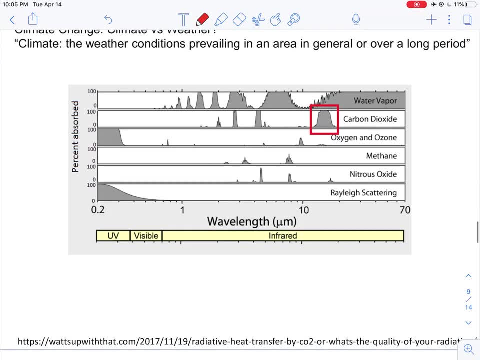 Right, So it's causing more global concerns, But it seems that there's really not much things we can do to stop this from happening. Okay, So another example I want to give about how human beings can influence the environment is the climate change. 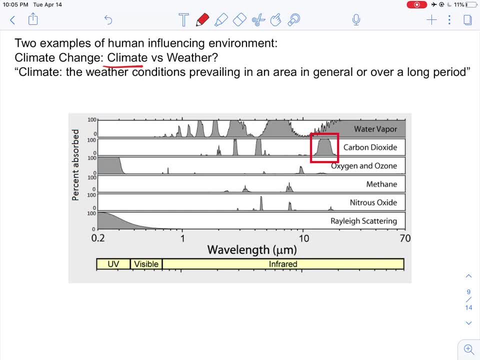 Okay, So we have been hearing a lot of debate on the climate change nowadays, Right? So we're seeing that some people are saying that, well, it's just the weather, Right? The weather can be cold, It can be warm. 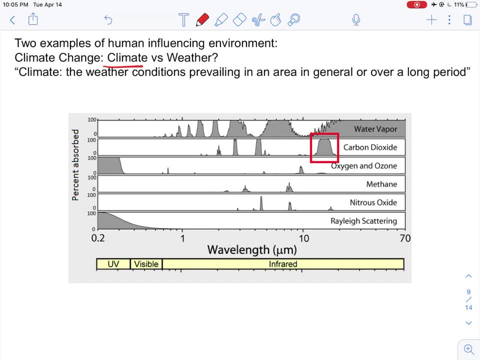 It can be. It can be anything, Right. For example, for the last winter, I think, we saw a few days that are very cold, but we also saw a few days that are really warm. Right, But we have to notice the difference. 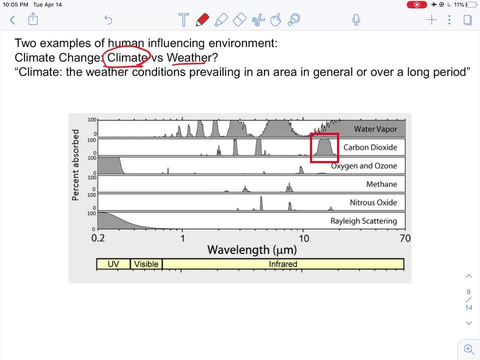 between the climate and weather. So whenever we talk about the climate, we're talking about the pattern or the feature or the trend of the global temperature in the year span, or in the time span of hundreds to thousands of years. Okay, But the weather? 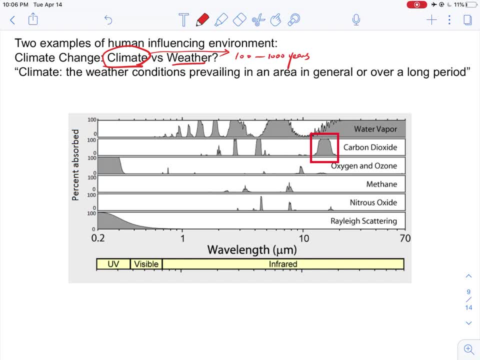 is just on a daily basis or even, for example, weekly spaces, Right? So if we track the global temperature in this longer time span, we can clearly see a trend that temperature is rapidly increasing in nowadays. Okay, So the reason why we're interested. 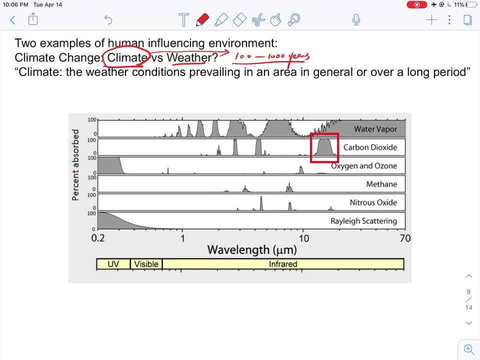 in the climate change is because people actually emitted a lot of greenhouse gas species into the atmosphere and then that's causing the warming of the global climate or of the global temperature, Right? So the reason why people stopped saying the term global warming is because 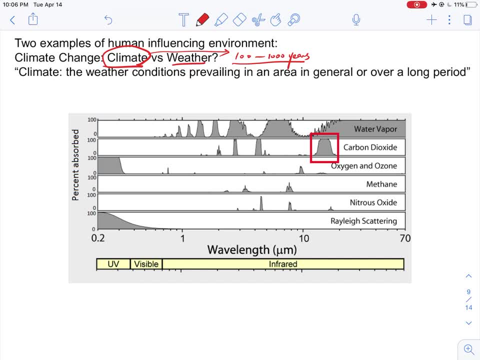 this average increase of the global temperature is not necessarily causing the global warming at each location, Right, For example, if we draw the Earth again, right? So temperature, if the temperature gets warmer in the polar region, then what that means is that 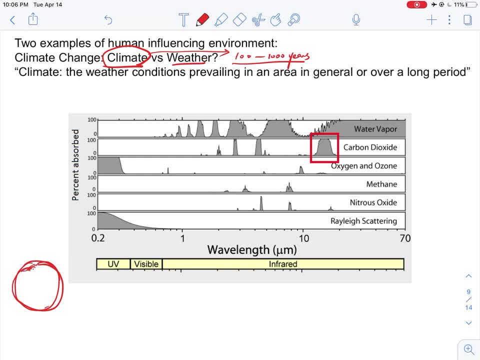 there's going to be more ice getting melted near the polar region. Okay, And we know that if the ice gets melted, it's going to absorb heat. So by absorbing heat, that's actually making the European countries cooler Right, Or making the southern 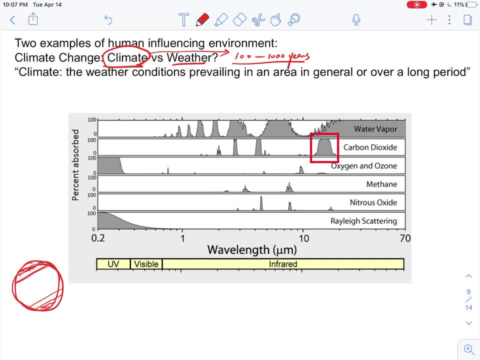 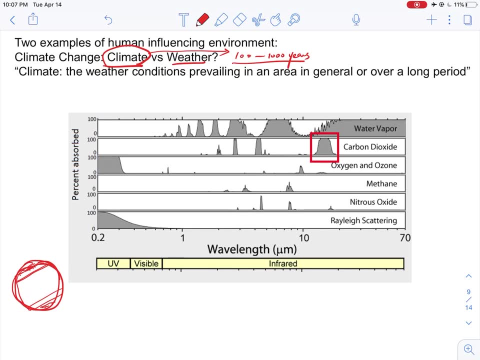 South America region or the southern Africa region. cooler there, But in terms of the global temperature the temperature is still warming, mainly because these greenhouse gas species are stopping or basically keeping the radiation or the infrared or the heating radiation within the Earth. here It's basically. 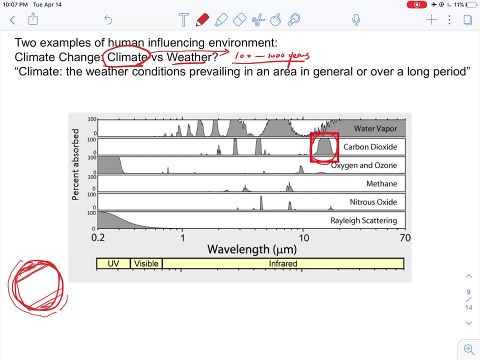 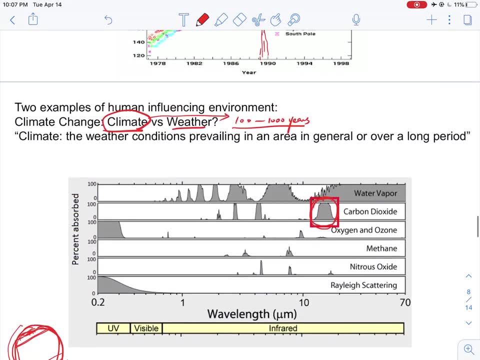 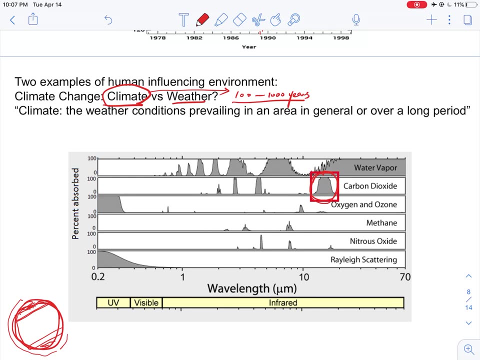 putting more clothes onto the Earth. right, It's trapping the energy within the Earth and that's going to cause this global climate change issue. So we're mostly interested in the carbon dioxide as the main reason or the main part of the global climate change. 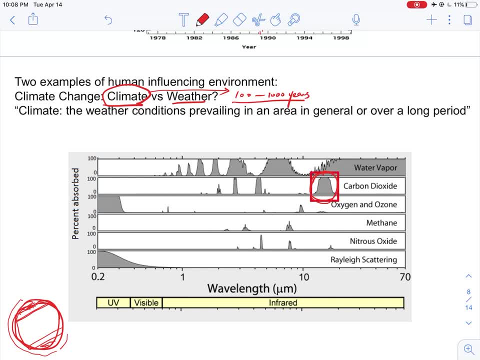 Because the carbon dioxide are being emitted in large quantities. right? Just think about the fossil fuel combustion. Everything is based on carbon, And once they combust them, they're going to form carbon dioxide in enormously large amount. right, And you can see. 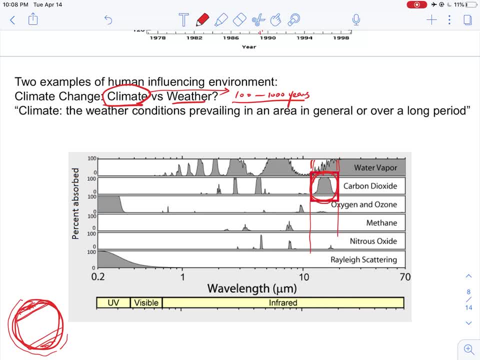 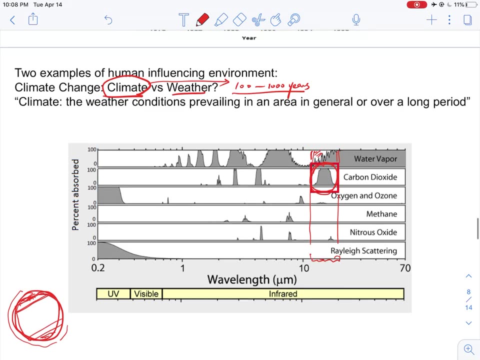 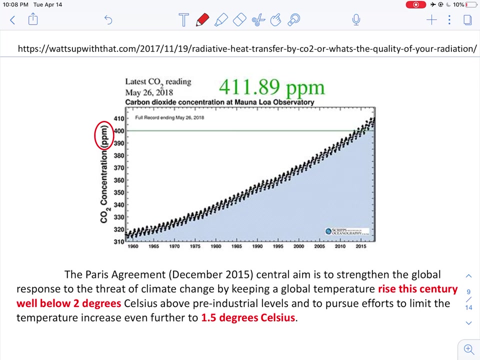 that carbon dioxide can absorb the heat in where the existing gas species cannot really absorb efficiently. So this is the heat that's kept in the atmosphere, right, And then, specifically for this bandwidth, it just represents the heat that's in the. 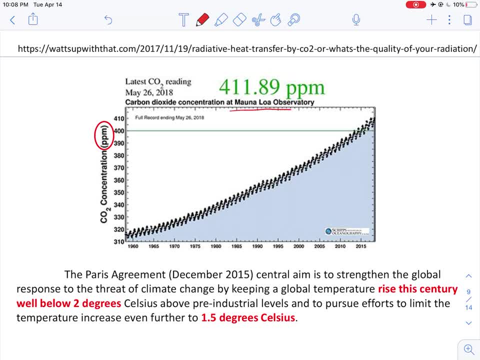 that's kept in the atmosphere, okay. So people have been tracking the concentration of the carbon dioxide for a long time, Right? So that's almost one-fifth or one-fourth of the existing concentration of the carbon dioxide. So 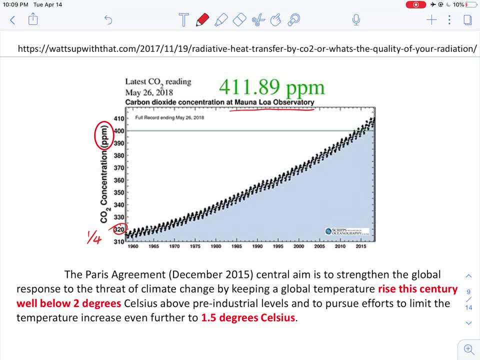 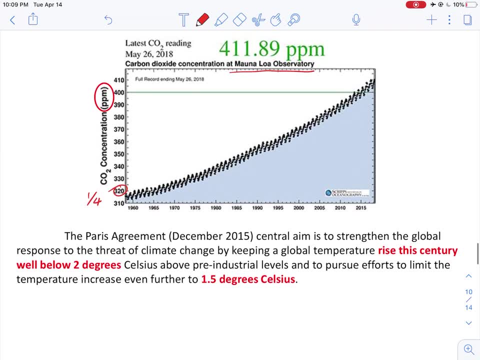 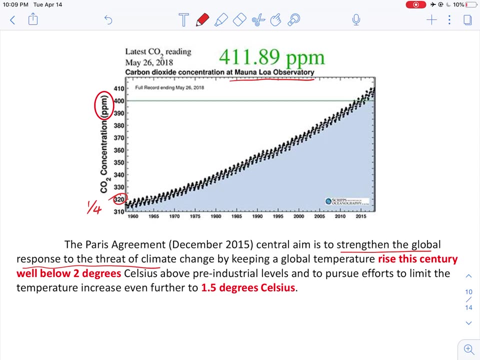 the carbon dioxide concentration is rapidly increasing and this is going to cause some global climate issues. So that's why, again, all the countries get together, because they notice that they have to do something And they want to keep the global temperature rise within. 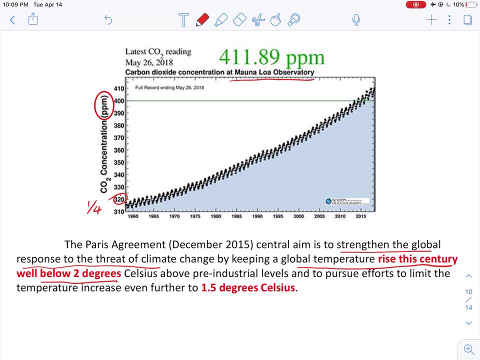 these countries to well below two degrees. Actually, two degrees means a lot, because if you think about the area where the average temperature is around zero Celsius, by increasing that temperature to two Celsius, then all the ice are going to get melted. So 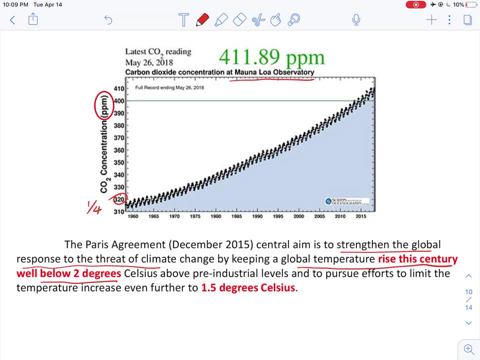 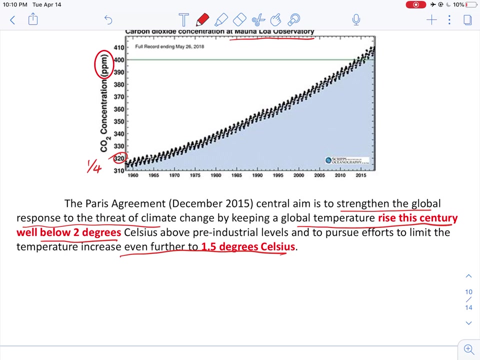 we're seeing more weather issues, for example, extreme weather. We're seeing more tornadoes or hurricanes in recent years, and that's potentially because of the global climate change. So the goal is to keep this global temperature rise to well below zero. 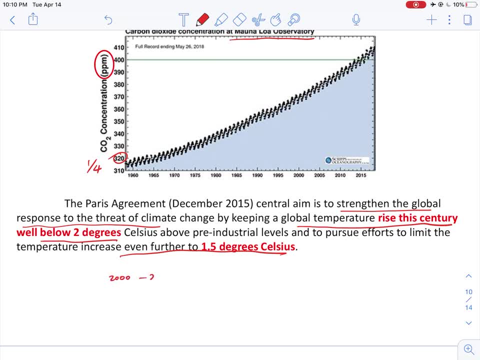 Celsius. So people notice that actually just from 2000 to 2018, so actually the temperature already increased by 1.2 Celsius. okay, which means that by just using 18 years we already finished all of our quota. 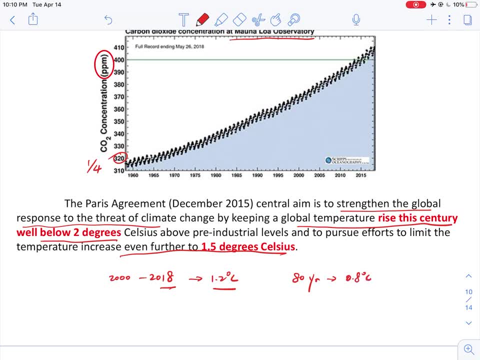 right. What that means is that for the global climate change, we're still relying on fossil fuel combustion. right? We can only see the consumption of these fossil fuels to be increasing, not decreasing, because- think about developing countries, for example Africa. 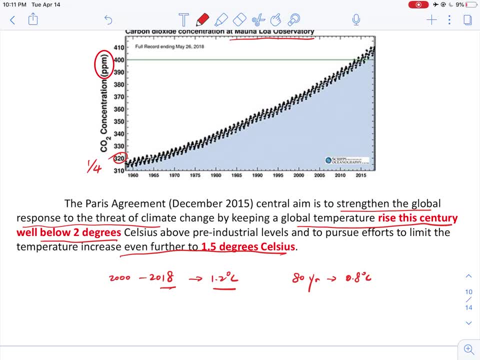 right. You only see the increase of these fossil fuel combustion and specifically right now, you can see that the oil price is very low, so a lot of countries are rapidly acquiring or purchasing these oil, and then it's good news for them. 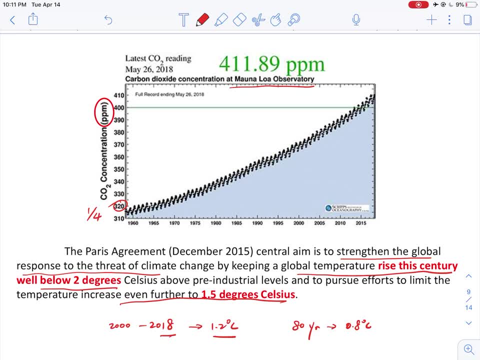 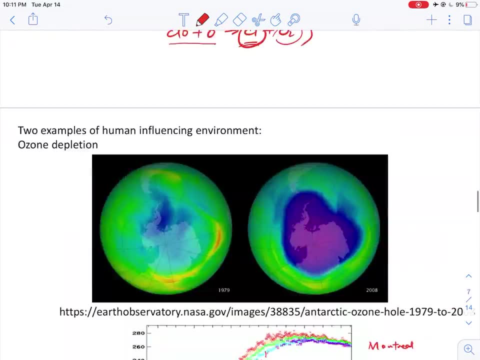 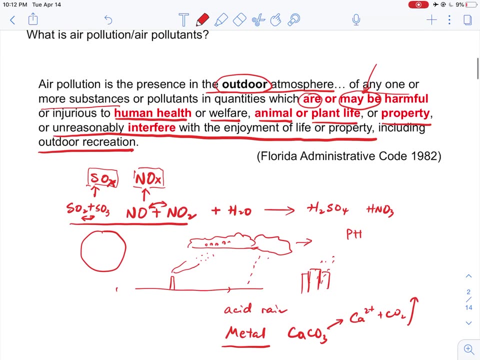 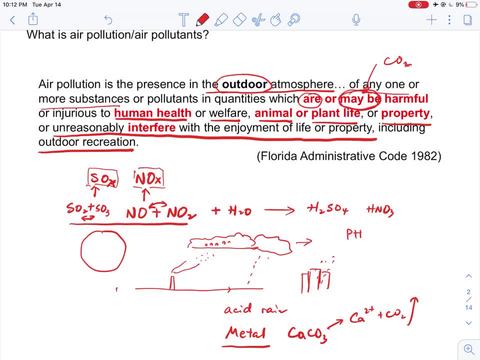 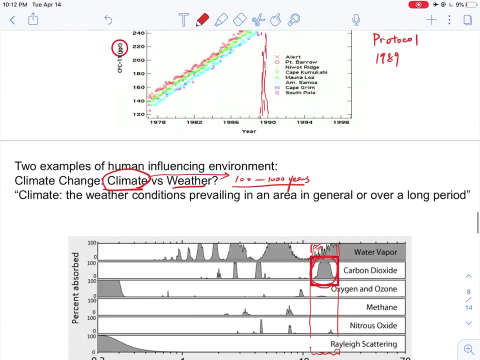 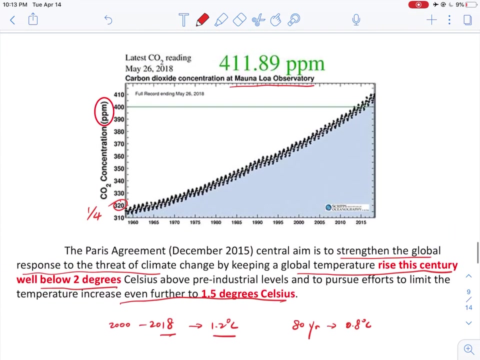 Thank you, Thank you, Thank you. This is my first talk about carbon dioxide, but I also know a bit about fossil fuel production as a result of massive impact on the global climate from the combustion sources. So I think we can just finish here in our class and we can further discuss further contents.